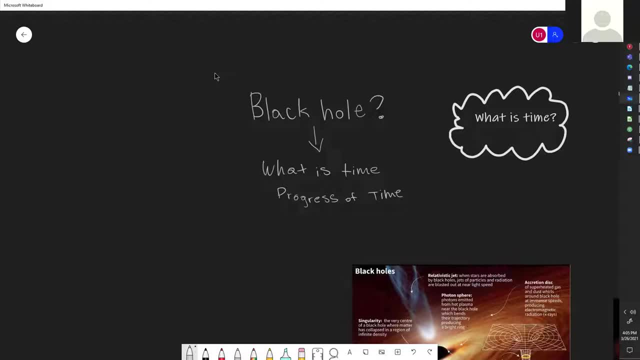 I was just going to say it's how we measure time. Okay, I was just going to say it's how we measure time. Okay, I was just going to say it's how we measure time, It's how we measure things and how we measure what's happening. 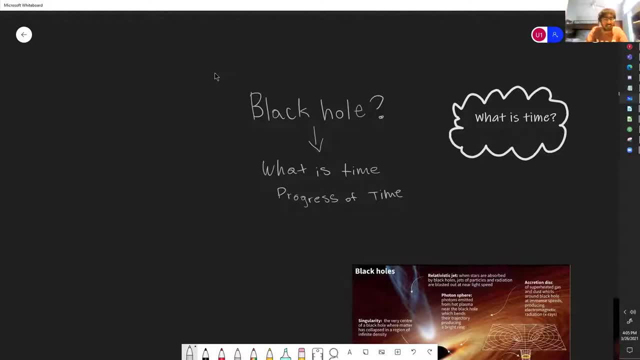 Let's go ahead. I mean, we do have units for time, right. We talk about minutes, hours, days, seconds, right? That's certainly true. Yeah, You give us a go, Jesh. What do you think time is? 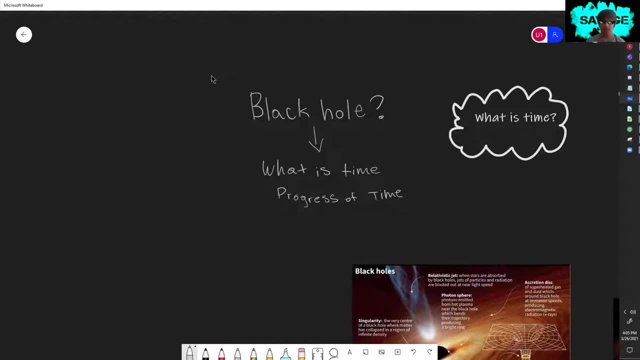 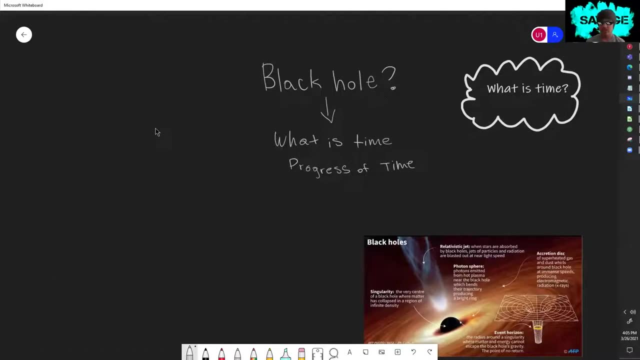 I think time is like. So basically a period, A period where like things are changing- Yeah, I mean like period- implies that there is an end and a beginning, and that's really not for time, right. 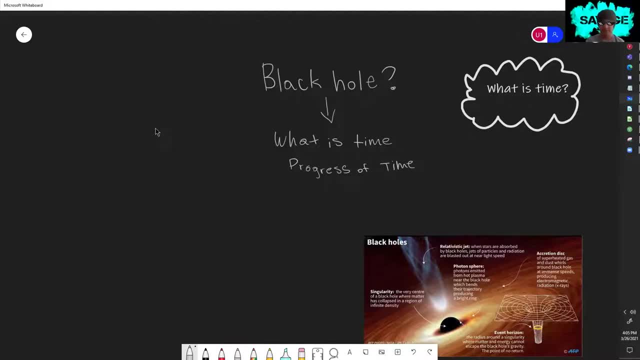 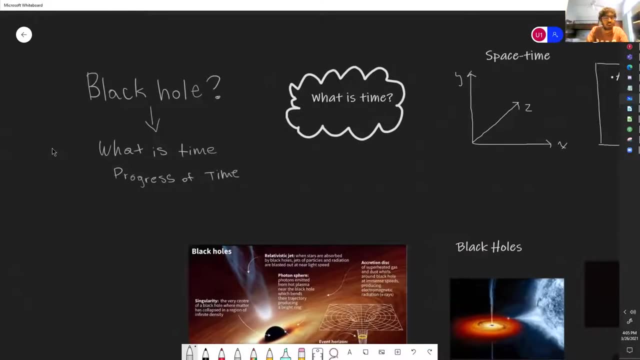 Time is Also: it's 405.. There's no boundary right. But yeah, time is basically how we're experiencing. change how we're measuring. change right, Like, if you run for 10 seconds, right, We're measuring how far you run in seconds. 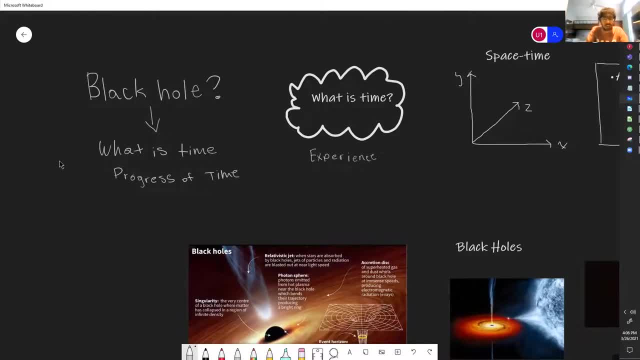 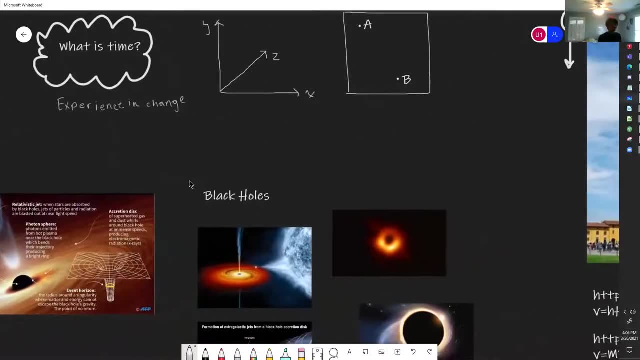 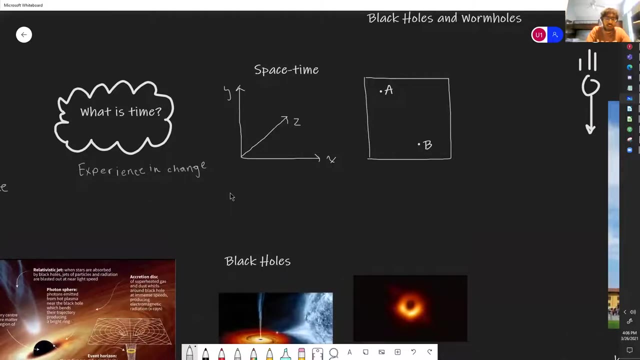 So we're using time to really measure how things are changing. Okay, Yeah, So, Siobhan GG. Yeah, It's already vague from the beginning. Okay, And then another question I want to ask is: how many dimensions do you think space is made of? 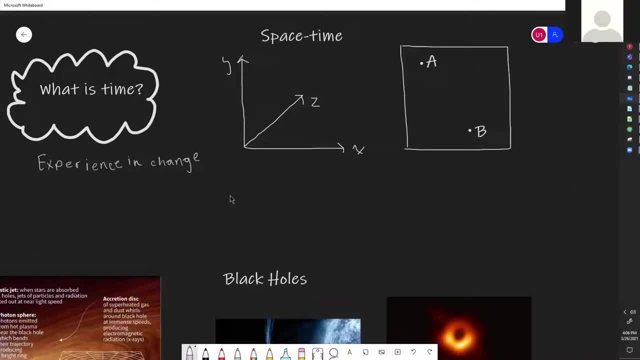 Four, Three, Four and three, okay, Okay, Ten, Five, Five, okay, Somebody said ten, Ten, Yup, Infinite. okay, That's Yeah, We have a lot of, We have a wide variety, Like maybe: 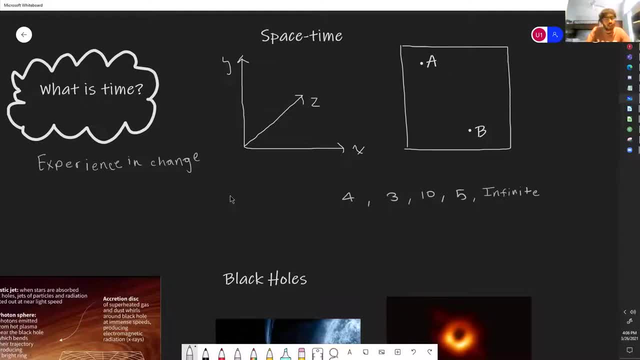 Yeah, Infinity, Yeah. So, as for humans, we can only really experience three dimensions. okay, Although some people argue maybe it's four, because it's a very common belief that time is the fourth dimension. However, that is not for certain. 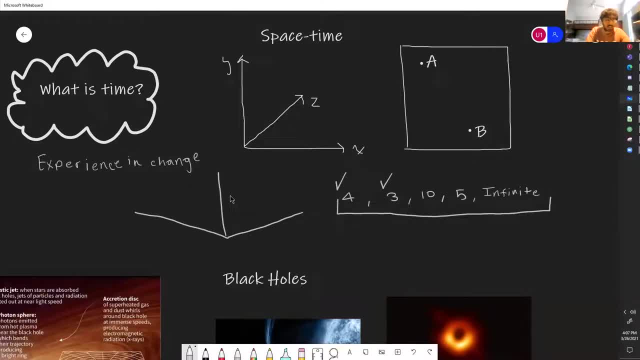 So we're just going to stick to the facts and we're just going to say there are three dimensions that we can experience. Okay, And so does anyone want to take a guess as to what the three dimensions, what they each represent? 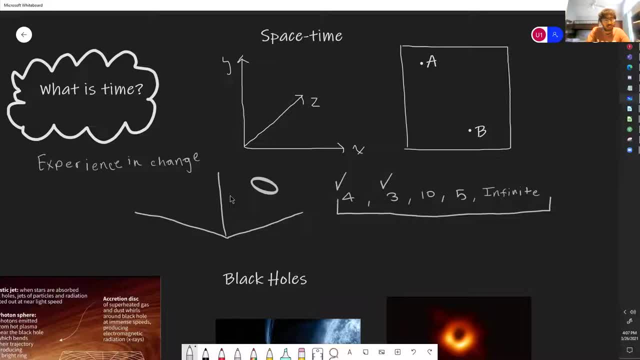 All right. So if you had a straight line, what does it have? Does it have length? Does it have width? Does it have height? Yeah, I heard Aram. He said length, width and height. Good job. 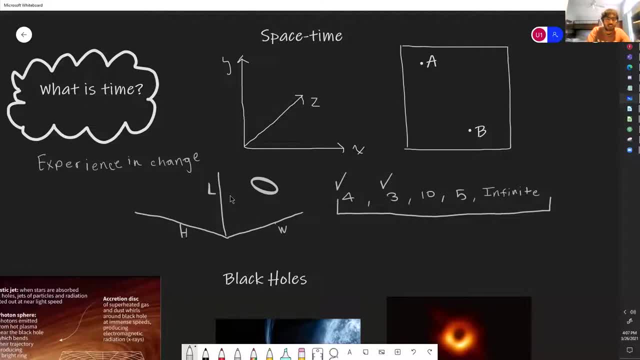 Yeah, Length, width and height, right. So like, if you look at this three-dimensional thing right as Audubon has kindly drawn, the x-axis kind of corresponds to length, The y-axis corresponds to height And the z-axis corresponds to width. 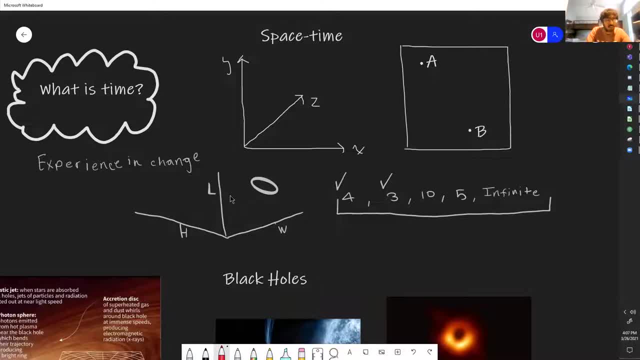 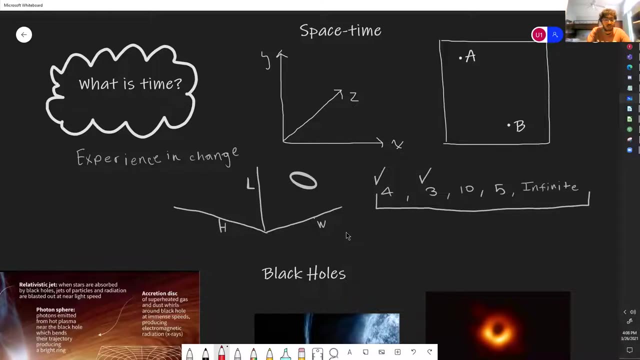 But of course we can always shift this around, So it's a very fluid thing. Okay, But according to some really popular theories, like, for example, there's a theory called the Clank-Kaluza theory, And they actually say that according to mathematics, there's two different numbers that could satisfy. 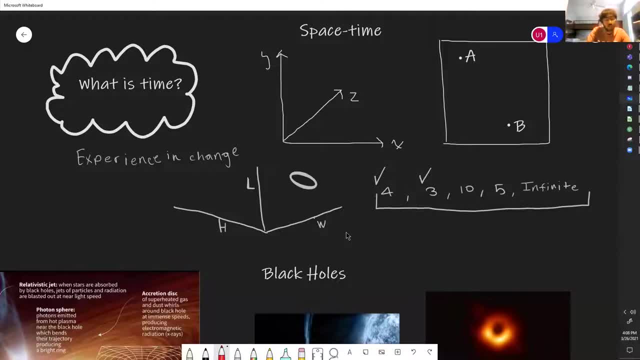 the universal requirements of dimensions. One is seven, one is ten. Right, But can we really experience all these seven dimensions and these ten dimensions? No, We can only see length, width and height. Therefore, that's why I call it the Clown Theory. 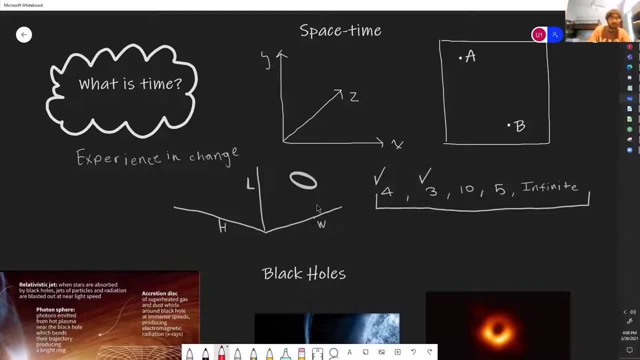 Yeah, And when we're talking about these extra dimensions, right, something that's really interesting is that some of these dimensions are like needlepoint, Like they're extremely small, So we can't even see them and we can't experience them. 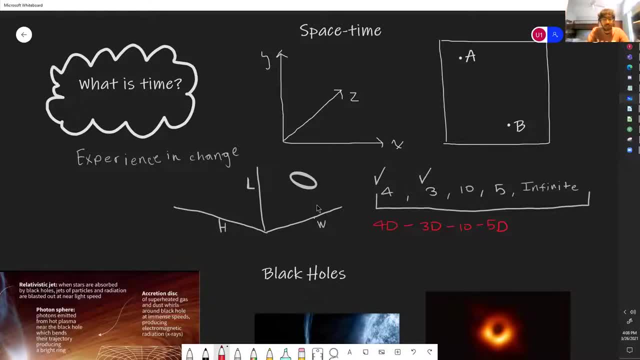 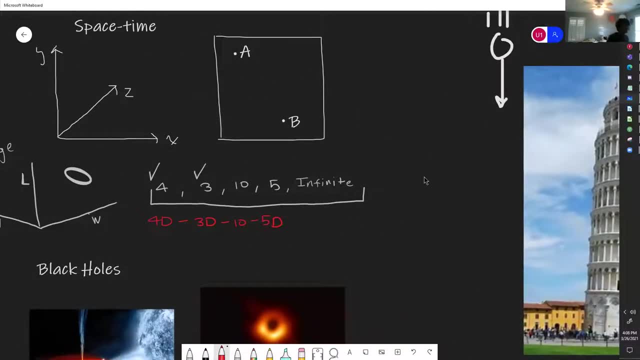 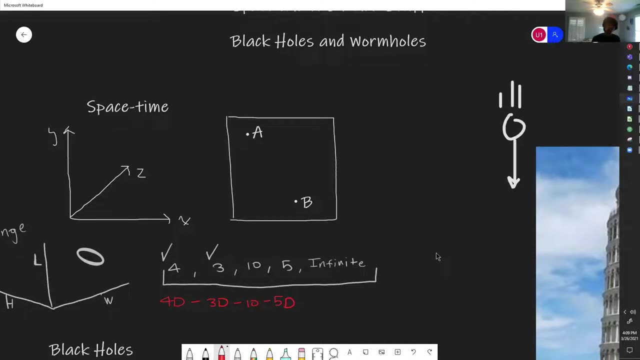 We can only experience these three, So I'm not sure how they did math to come up with eleven, but that's math, That's math, That's math. So any questions so far? Yeah, all of this is going to be a little vague, but it's fun. 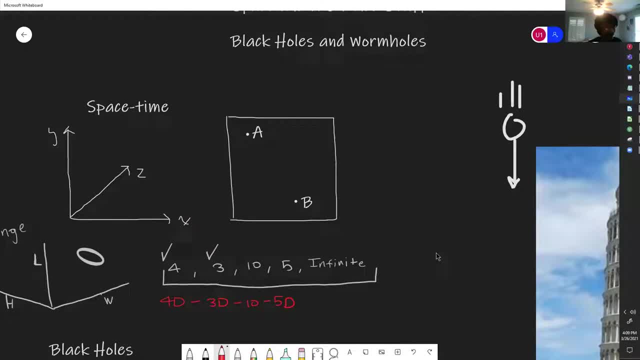 It's interesting. It's interesting how scientists come up with these weird answers, And that is why we joke about scientists all the time, And this is why I only. Isn't there supposed to be four dimensions according to the general laws of astrophysics? 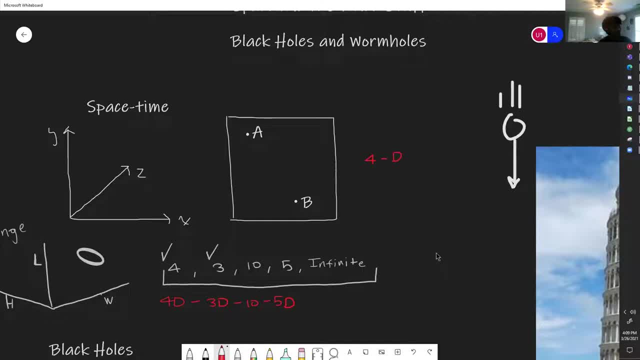 Well, yes, There's supposed to be four, But other scientists disagree with that And other scientists think there's more than four. There's no commonly accepted like, It hasn't been completely proven like mathematically, if the fourth dimension 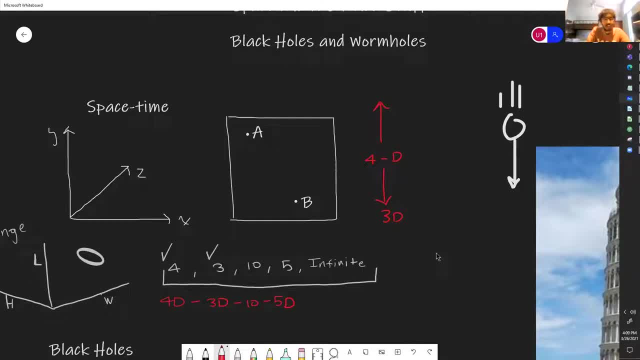 If it is time, right, Like some people think it is time. Mathematically it's been proven like there's more than four. definitely, But what does the fourth dimension really represent? No one really knows How can there be more than four dimensions? 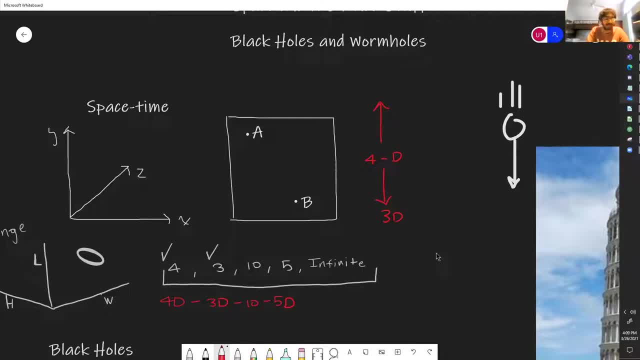 Don't ask me. I didn't come up with these math. Yeah, you know. now I'm starting to question Why the theaters aren't calling the movies four dimensions, Because like it takes time watching a movie and like you get 3D right. 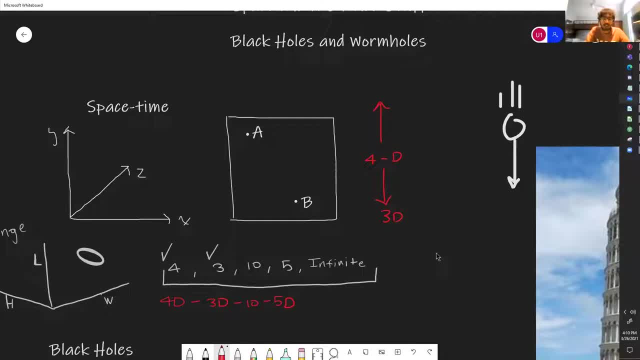 So boom. Or perhaps it's like with senses: right, It also incorporates your senses into the experience. Yeah, but I just got the million-dollar marketing proposal right there. Just make Just call all 3D movies 4D from now. 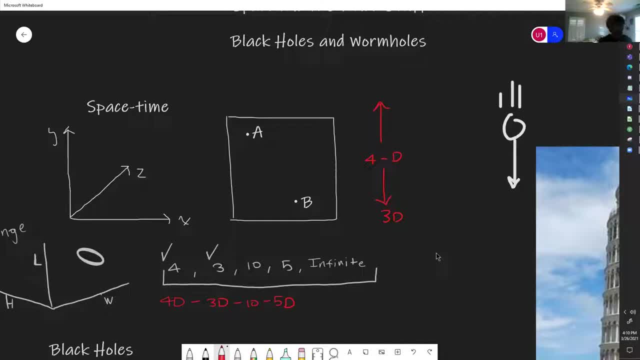 Boom, There you go. Yeah, Yeah, And so Everybody. 4D movies for sale. Yeah, I know, Right. So Before we move any further, right, I want to establish a concept of space-time, right? 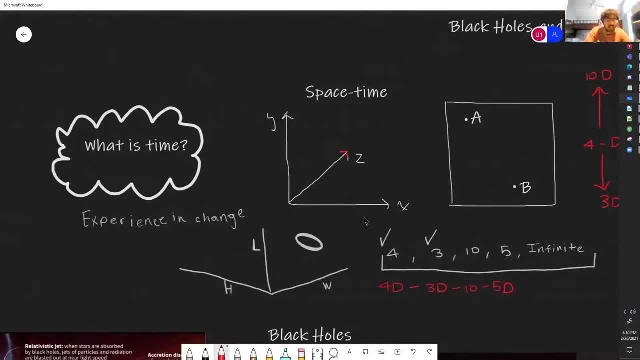 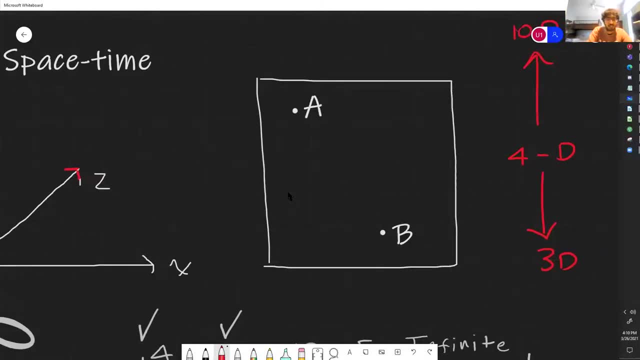 So space-time is really just this idea that you can't separate change and time, right If you? So if, Audubon, if you move to that rectangle with the A and B right. So here's a question. 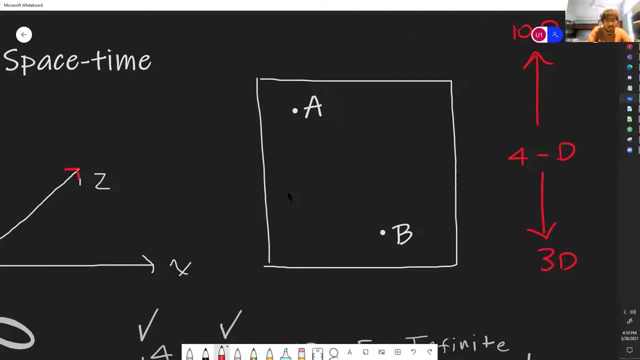 Could you get from point A to point B without any change in time? No, right, Because it's Your position is changing. Your position is changing while you're traveling from point A to point B, right? So what this really demonstrates is that you can't separate time from space, because 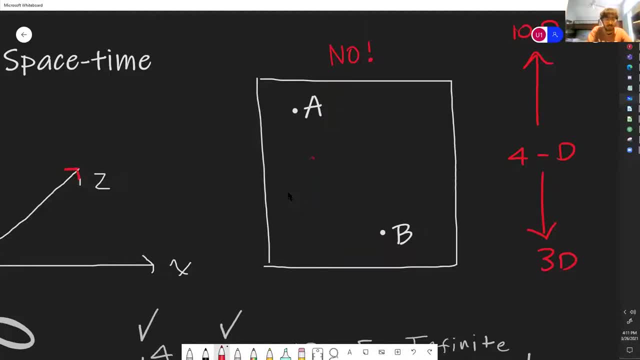 any change in space is measured in time. So this is how scientists- I think this is the logic-ish. There's also some math, but this is kind of how we think of space-time. right, You can just imagine space-time as like a piece of fabric, okay, 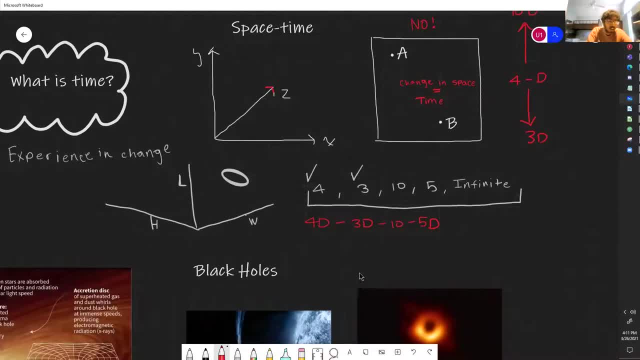 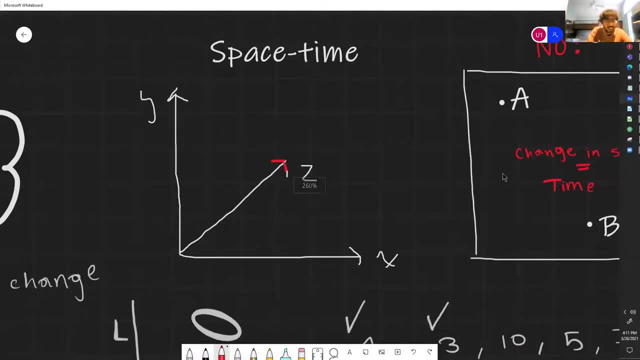 And any change of a point on space-time is going to result in a change in time. okay, So it's. I know it's a really, really vague definition, vague description, but I hope all of you get it Yeah. 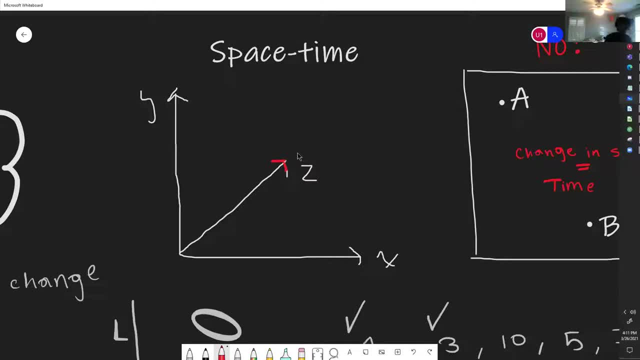 Any questions about space-time? I think Jesh does. so, Jesh, Speaking of space-time, do they have like time in space And if so, like? is it the same as the time here on Earth, Or like? 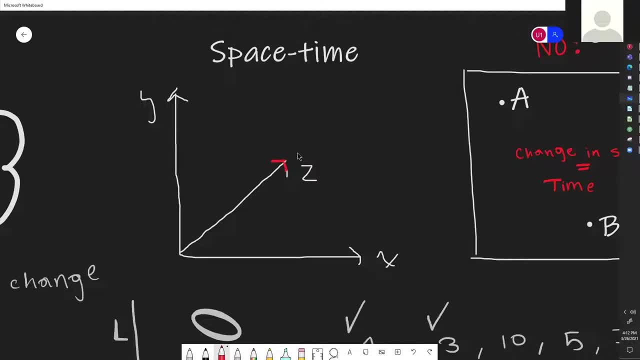 Is it like: Like what's the speed of time in space? I don't know. So the speed of time is not constant. actually, The speed of time is relative. So if you are going at, for example, 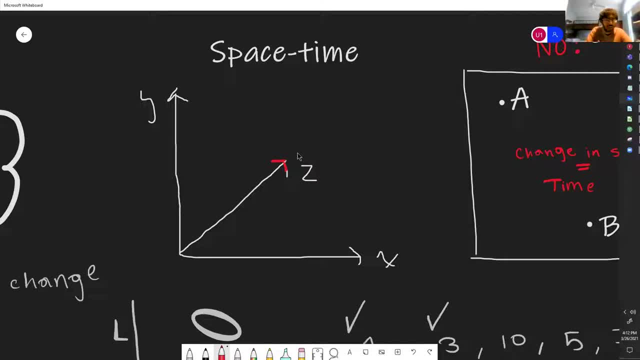 If you had two cars, right, One car is going at 10 miles an hour and the other one is going at, let's say, a quarter of the speed of light. right, The car that's going at the quarter of speed of light? 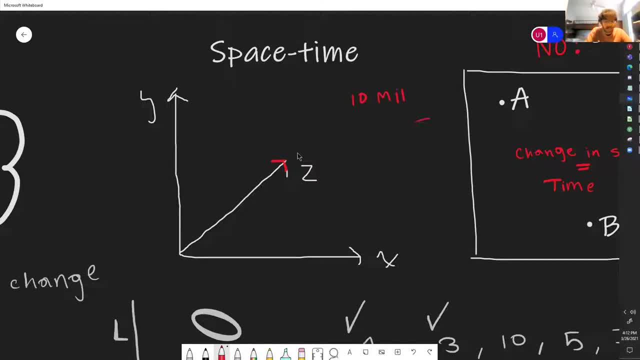 Is actually going to cover the same amount of distance, right? If they're on like a 10-mile track, It'll cover that 10 miles in less time than that car that's going 10 miles an hour. So time is very relative when you're talking about fast speeds versus slow speeds. 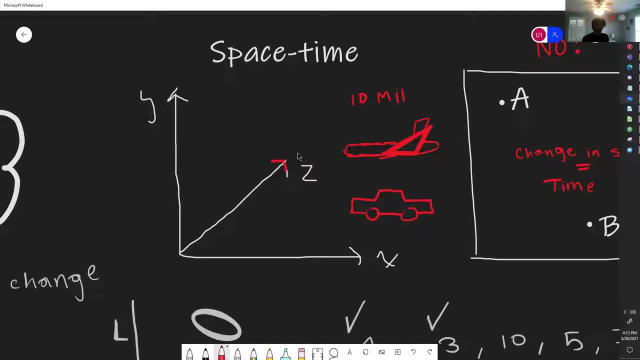 I think the example on the whiteboard of airplanes and planes also explains that right. You think, You would think the airplane going fast, you would feel the airplane going at 600 miles an hour. But do we feel the airplane going at 600 miles an hour? 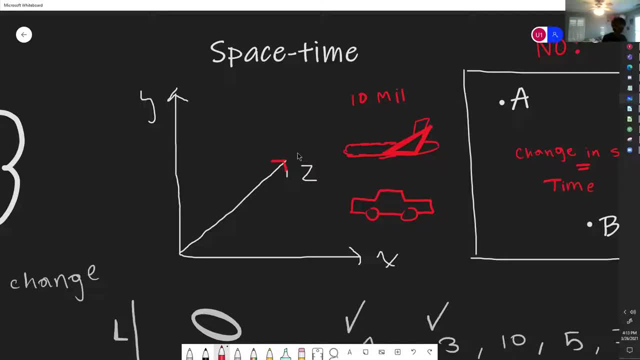 No, we don't, Because we literally see outside the window and see like three clouds slowly going along. But guess what, When you're on the ground, you're going like a tenth of the speed of the airplane, But you still feel like you're going faster, right? 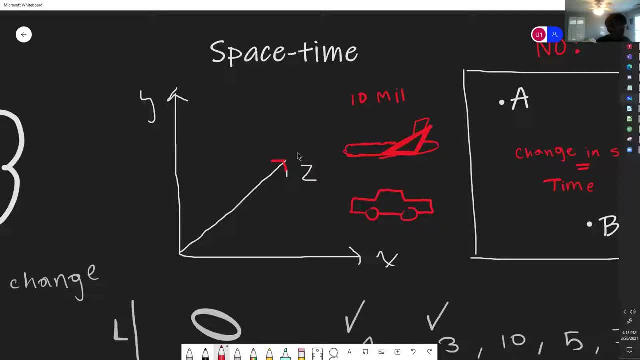 So Speed and time are very relative in terms of feeling. I think that also plays with how I felt procrastinating through spring break. So it was very relative. Even though everybody had the same time, I felt like I wasted most of my time. 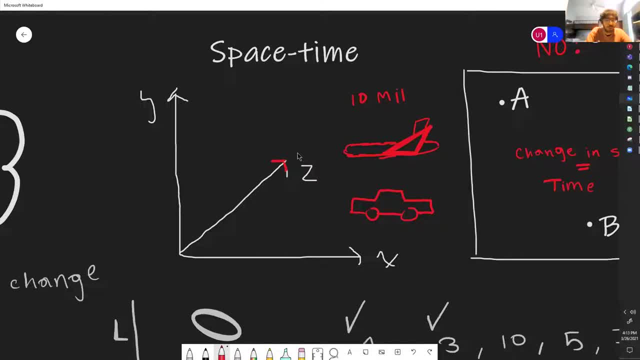 Therefore it went by. When you're having fun, time seems to be going by really fast, right, And when you're bored, it seems to be going by super slow. Exactly. So time is really really relative, It's not a fixed quantity. 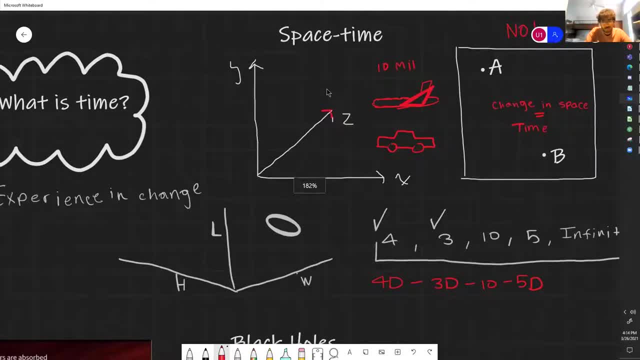 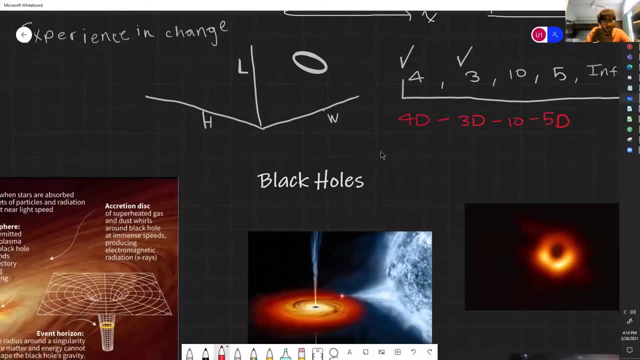 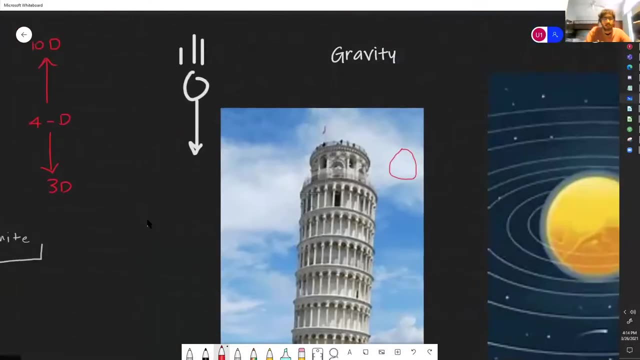 Okay, So any questions about space-time before we move on? No, Okay, Well, now let's move on to gravity. Other way To the right. Yes, So all gravity is is, You know, actually One second. 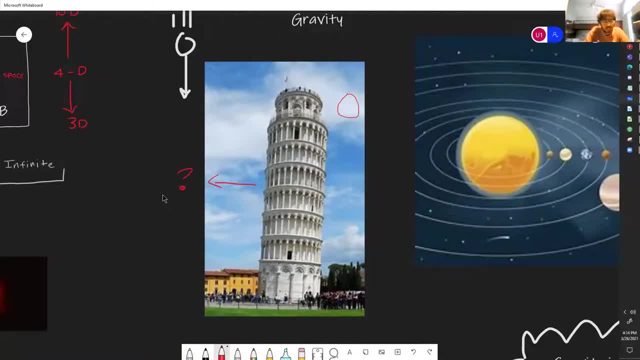 Before we start talking about exactly what gravity is, I have a question for you. Okay, Does anyone recognize this tower? Yes, What's it called? The Leading Tower of Pisa, Pizza, Pizza. Who can spell the last word correctly? 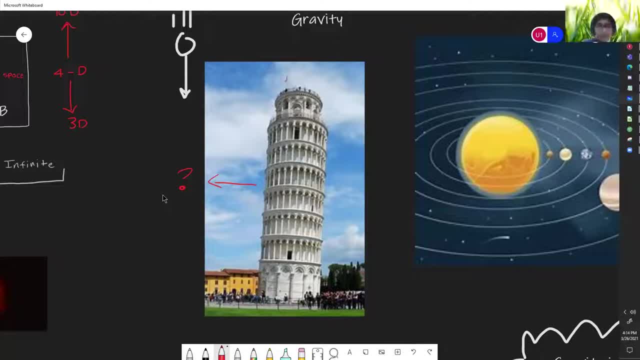 You get a million bucks P-I-S-A. The Tower of Pisa. It is the Leading Tower of Pisa. Okay, So if we took a bowling ball to the top of the Leading Tower of Pizza or Pisa, sorry. 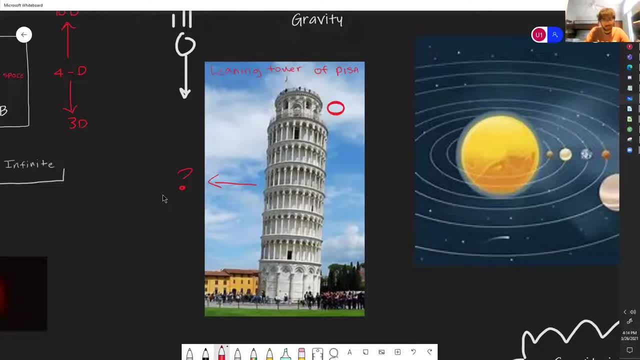 and we dropped it. Which direction would the ball go? The one it's leading toward Down. It would go down right, Because for us the force of gravity is downwards, Because gravity tries to go toward basically the center of any object, what we call the 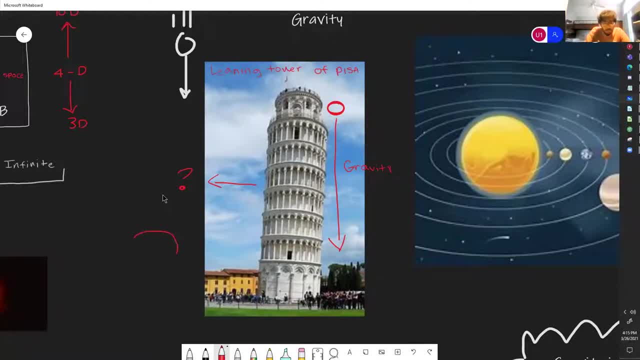 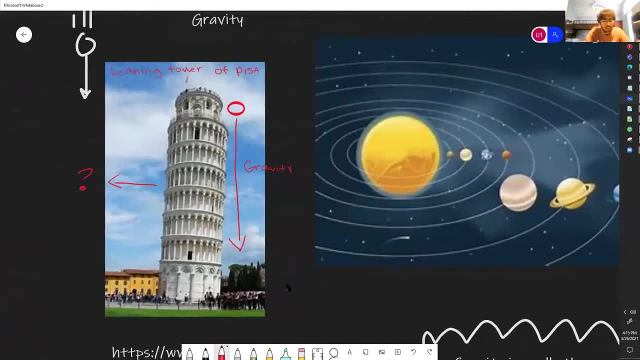 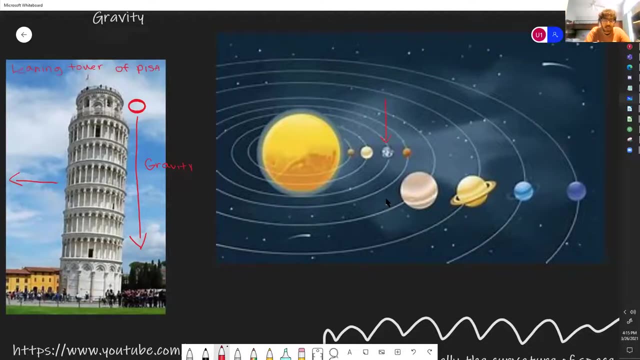 center of mass, Okay. But if you look at the solar system, for example, you would think, okay, gravity is pointing straight down on Earth, so it must be pointing straight down for all these planets. But that's not true. So here's a question. 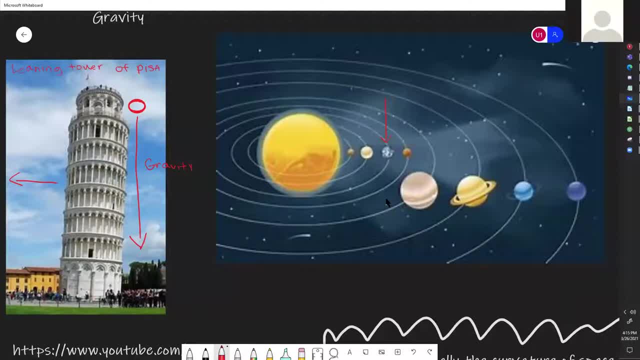 What keeps all the planets in orbit? The sun, The sun, The sun. And is the sun below the Earth? Is the sun below Venus? No, No right. It's basically pointed inward to the circle. So the force of gravity in the solar system is not down, but it's actually toward the 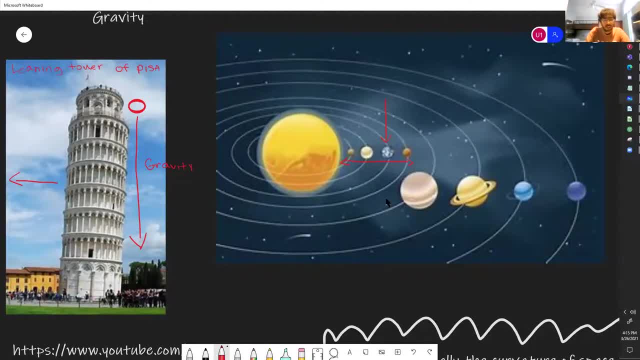 sun, Because the sun is the center of mass for the solar system. Okay, The sun is down for Pluto For sometimes, Yeah, For some, yeah. Some planets are not on a, they're on a more of a elevated axis. 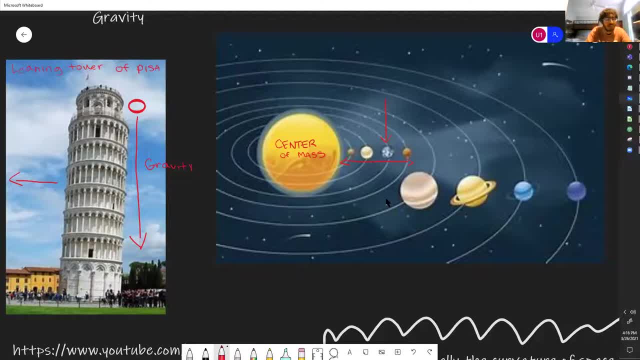 So they're sometimes below, sometimes above, But in general we can just imagine that they're all on a straight line, Okay, Like on the same plane. So gravity is actually in this case, instead of pointing down like we would expect, how. 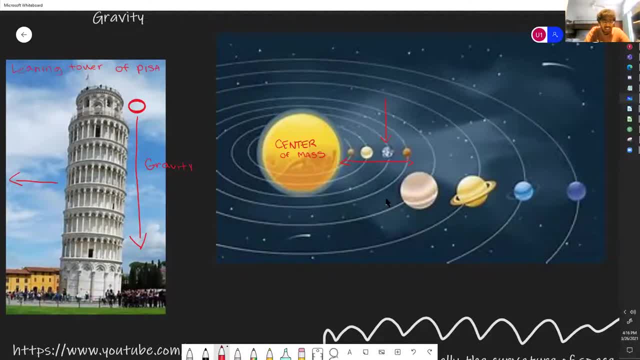 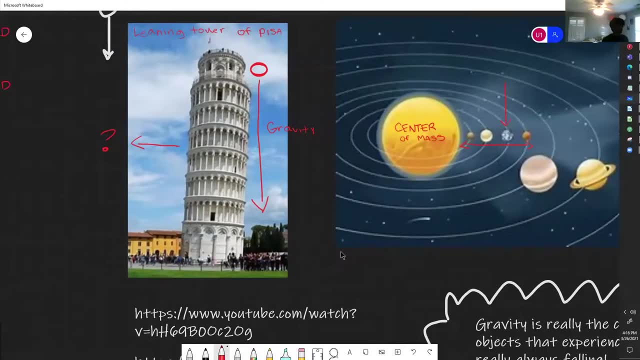 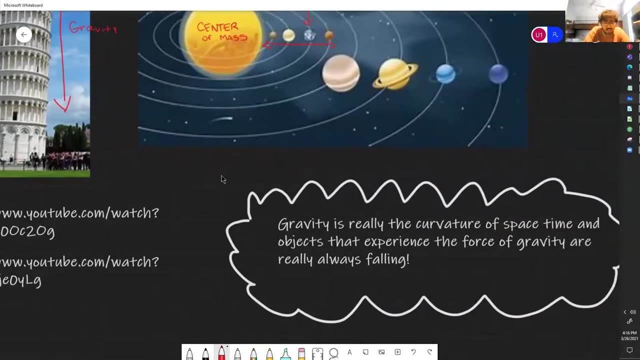 it is on Earth, it's pointing toward the sun, And let's take a look at why exactly this is. Okay, That was weird. So before we move on, I want to basically give a description of gravity. All gravity is is a curvature of space-time. 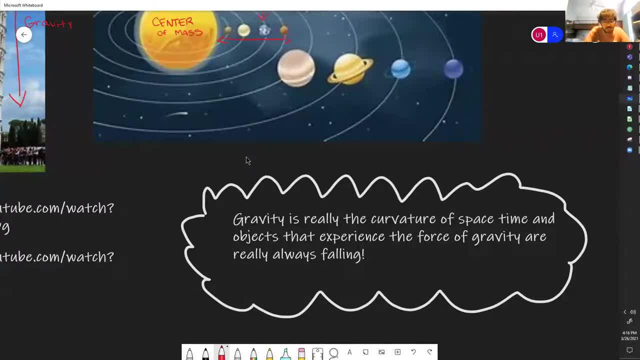 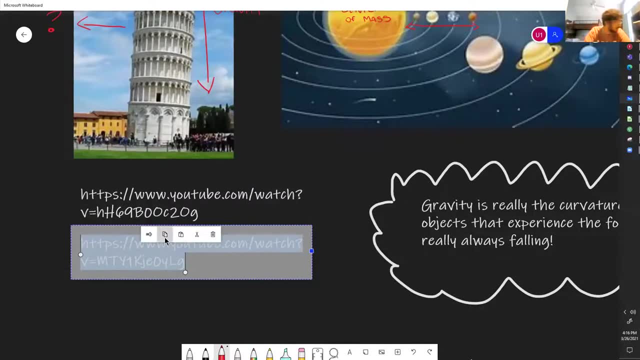 And we're going to look at an animation and an experiment by a professor to really dig into that definition. Okay, So just keep in mind that gravity is a curvature of space-time. Who's calling me So one moment as I load. 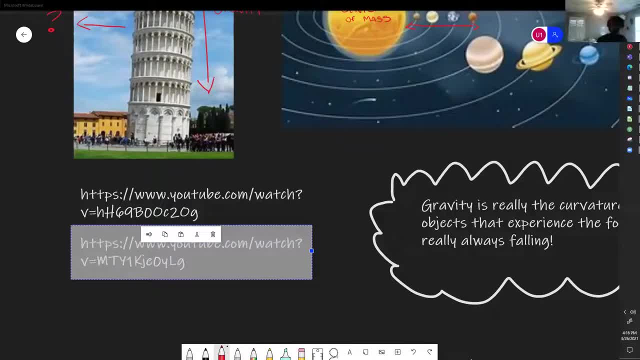 Can you copy? can I only copy one link at a time? Yeah, No, if you use a clipboard extension on Windows, you can get multiple links. So do you guys? This is a demonstration by a professor of gravity. Okay, 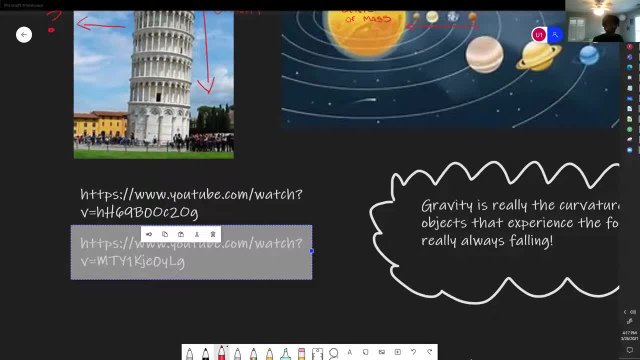 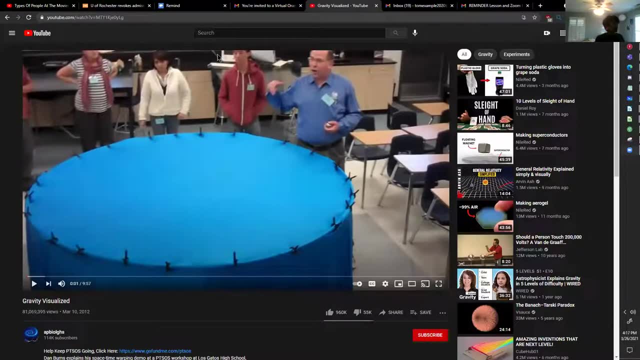 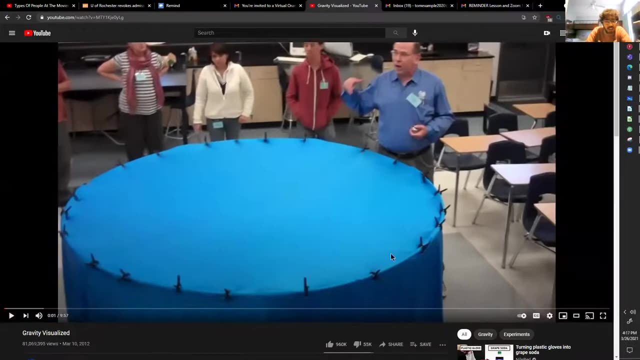 So what we have here is actually a sheet of spandex that has been stretched so that it's straight. Okay, So we can imagine this as space-time with no objects, no mass on it. Okay, But once you put mass, it actually causes it to curve. 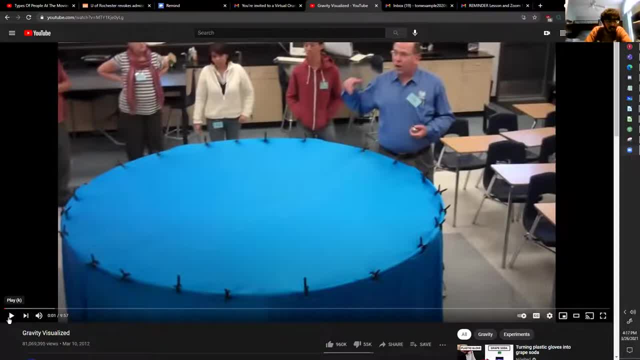 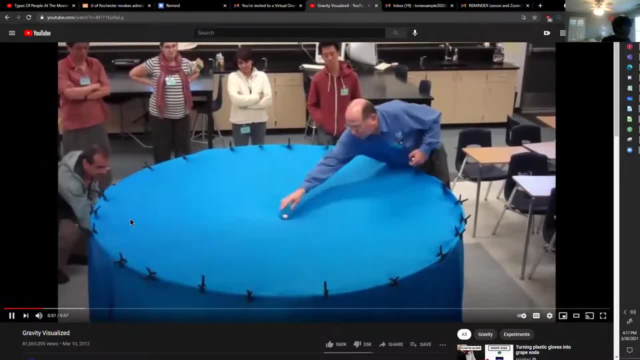 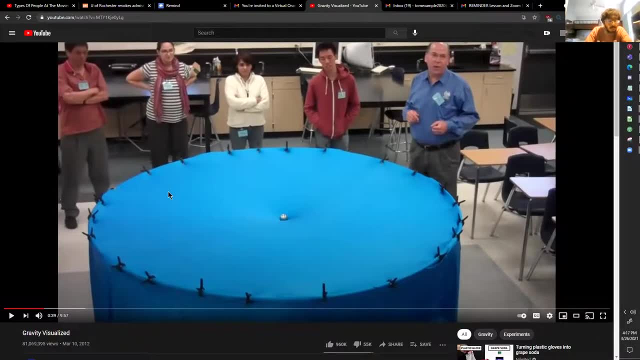 Oh yeah, Oh yeah, Oh yeah. So you put matter. So we are going to be putting masses right, Because any corporeal object, any piece, any solid object, right, Even air has mass and it's made of matter, right. 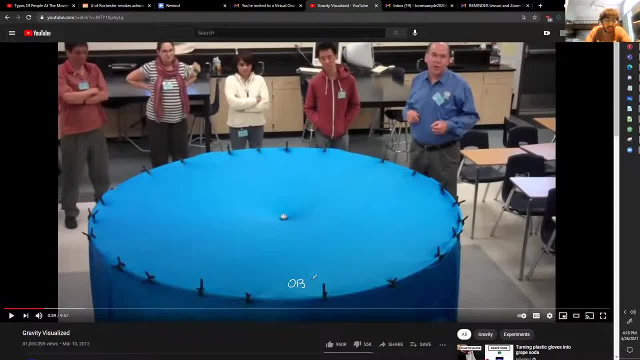 So whenever there's matter and mass, it's actually going to cause space-time to bend right. So, as we look in this demonstration, space-time was originally flat, But once we put this mass into the center, what happened to the spandex around it? it curved. it curved downwards right instead- curvature. 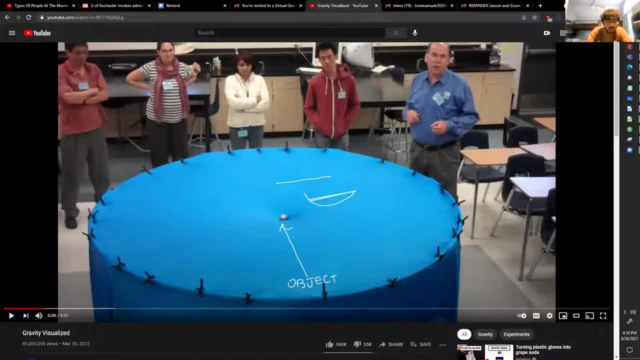 downwards of space-time. that all that really is is that's gravity, that's what makes things fall, okay, so any questions about that? so far, everyone getting it. okay. so far, yeah, everyone. uh, let's, let's hope the brains didn't go too much, just just yet, yeah, okay, so. 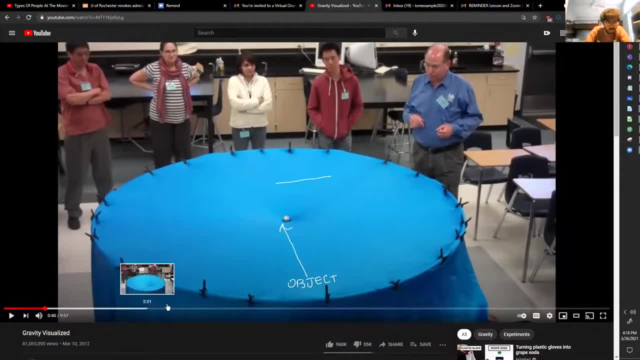 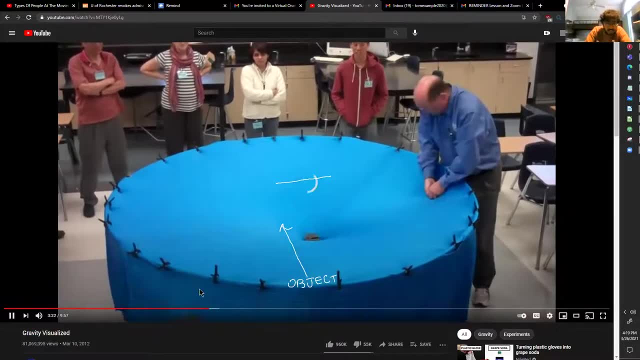 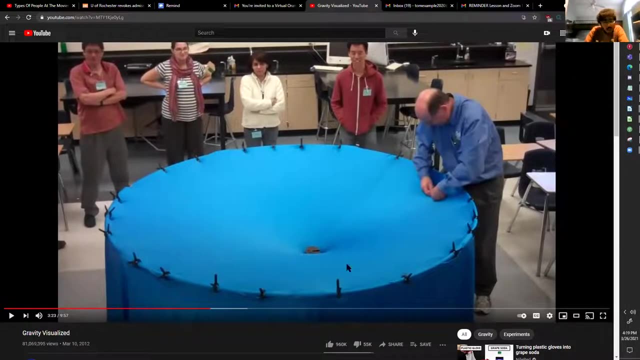 let's skip ahead to around. i think four minutes, okay, yeah, okay, yeah. so let's back up like 10 seconds or so. so what we have here is now we're going to put a heavy mass in the center, right, and so now we're going to kind of demonstrate the orbits. of objects due to the gravity of the object, so we're going to put a heavy mass in the center. so what we have here is: now we're going to put a heavy mass in the center right, and so now we're going to put a heavy mass in the center right, and so now we're going to put a heavy mass in the center. 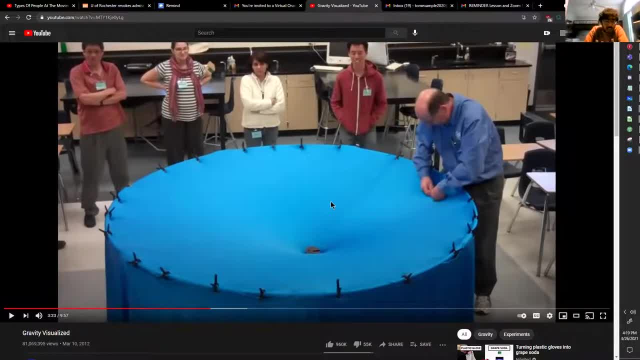 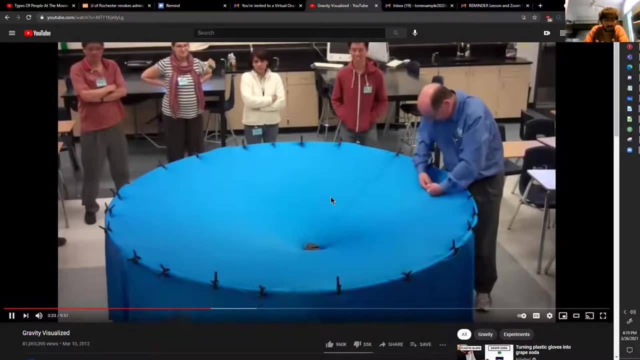 to gravity. okay, so what's actually going to happen is this professor is going to release some small balls and observe what happens to the balls when they get near that, near to the mass, when the spandex is curving downwards. okay, observe what happens, and so i have slightly more in one. 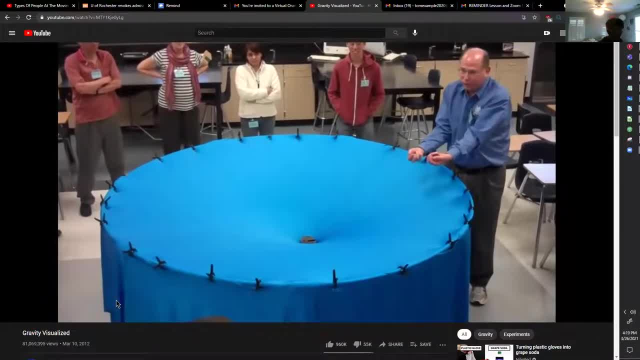 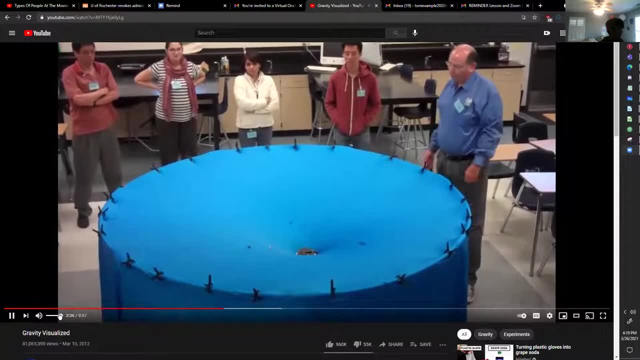 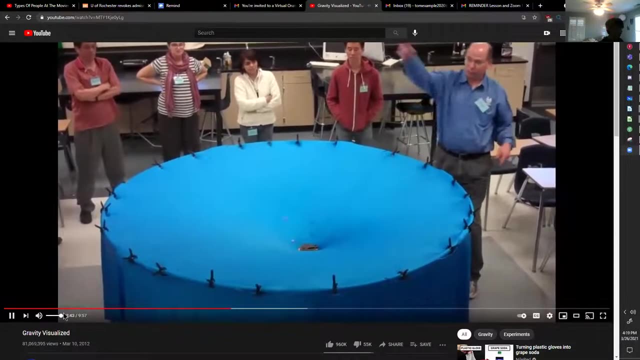 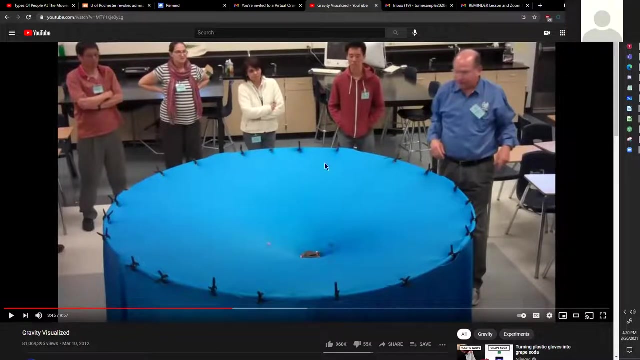 hand and another vital conscious to do that. you want to get it to be spread out a little and just there's a light and the balls curved toward the center where the big mass was curving down. yeah, they curved to the center, right, some balls went directly toward the center like they went directly to the mass, so they. 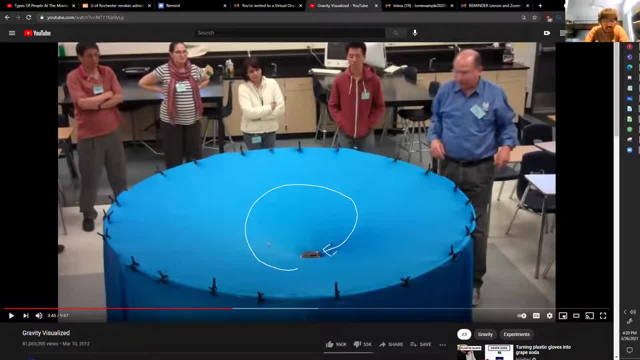 curved a tiny bit, but they ended up in the mass almost instantly. but some balls actually went in a bunch of circles before they went and joined the mass in the center right, and so this is basically how orbits are working. so the force of gravity actually has to be balanced with the rotational 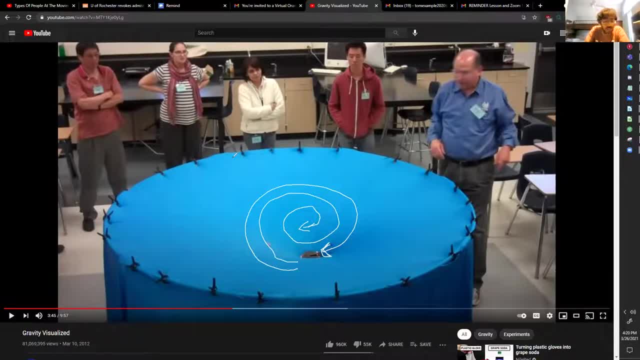 force of objects. so the planets are actually moving at a certain speed, at certain distances, uh, at certain distances that cause them to basically stay there. it makes sure that the they don't go toward the mass. okay, so this is really how orbits are working. okay, so this is really how orbits are working. 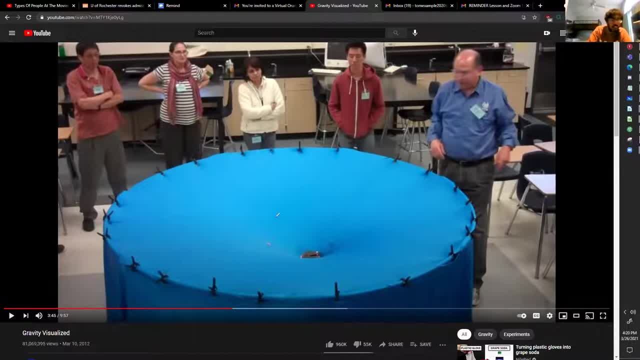 orbital motion is working. these are just. they're going around the edge of the curvature, so they're kind of falling inward, but then they're also being pushed out on the opposite side, right. so on one side they're kind of curving inwards and then they go close and then they're. 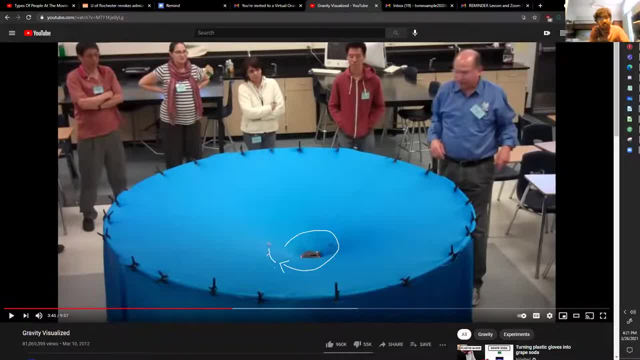 being and then, due to their speed, they're also leaving and then coming back in. so this is basically how planets are orbiting, okay, and this is also that- that nature of uh partly going in and out, inward and then coming outward- is why our orbit is in a perfect circle. 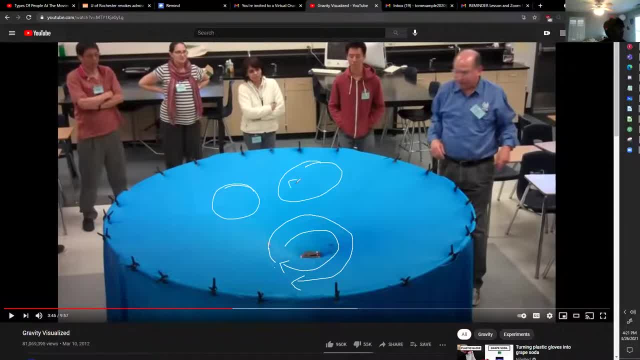 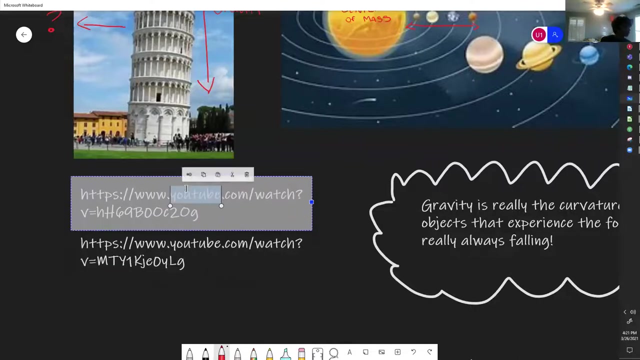 and it's more like an ellipse. is an ellipse, yeah, it's like an oval, okay, yeah, so any questions about this? brain's not mush yet. good, brain's not mushy yet, yes, and so now let's look at the second animation. so this was the simple animation. hold up, the second animation is not going to make it's. 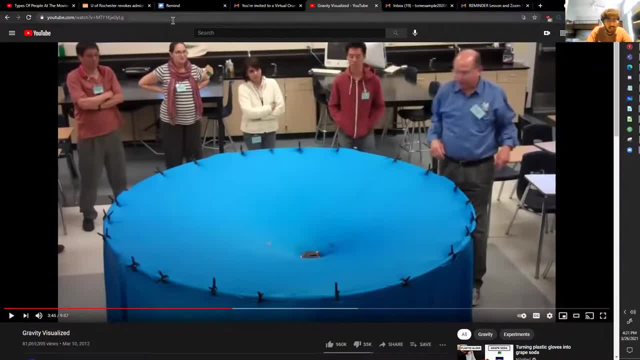 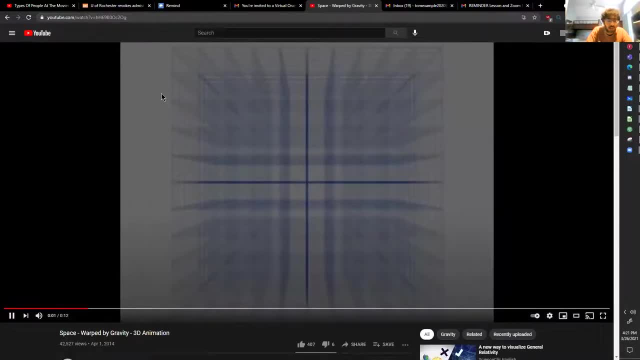 not going to. this one is a more realistic. this one is a 4d animation of gravity and observe what happens when the ball comes through. so this is really fast, so pay attention. so what happened when the ball went through that cube of space? it bended, yeah, it bent right, so that mass basically kind of curved. all of these. 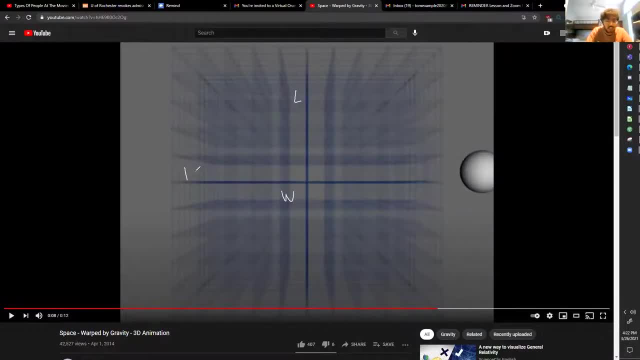 lines that we used to generalize space-time. it actually curved it toward itself- or sorry, not toward itself. it kind of curved outward right, and so this is a more realistic representation of what happens, but it's really difficult to understand, which is why we like to use 2d. 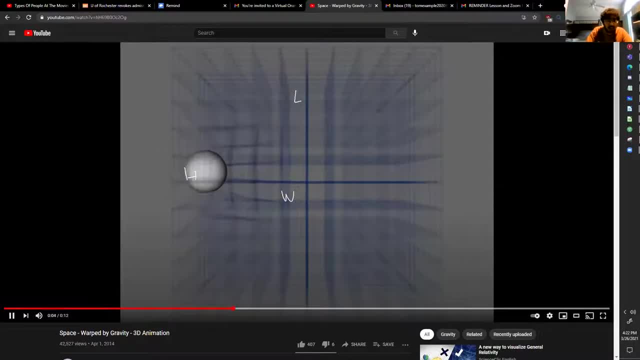 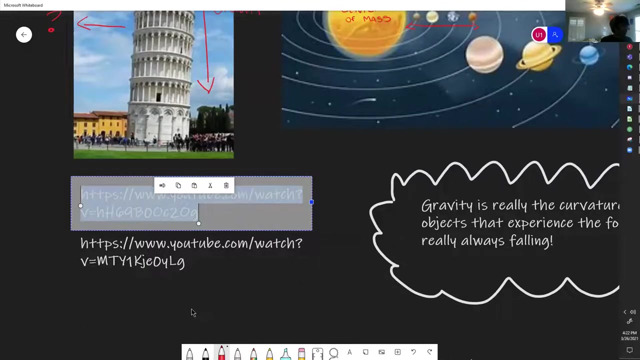 approximations, like with that span representation index sheet. okay. so it's really kind of pushing it away a little, making these little curves, and these curves are what we experience. that's gravity, okay. so any questions about gravity before we move on? y'all are doing great. uh, let me put the whiteboard back on, all right. yep, it's back. so. 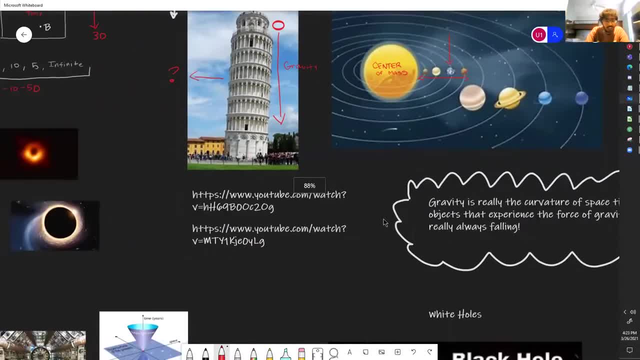 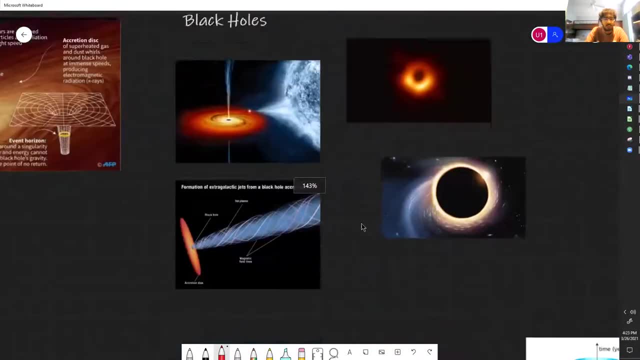 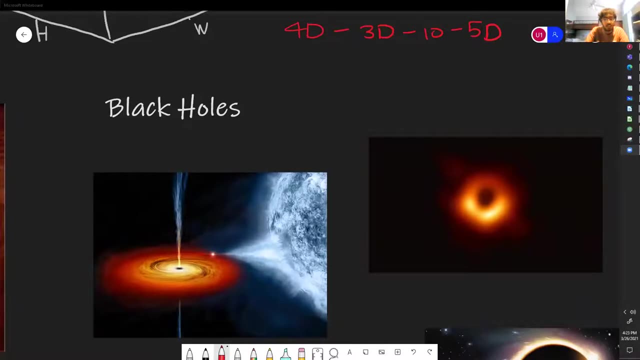 now we've established the basics of what we need to know. now we get to move on to fun stuff. now let's move on to black holes. so do you guys know where a black hole comes from? like what object turns into a black hole? a star, a dead star? a star, yes. 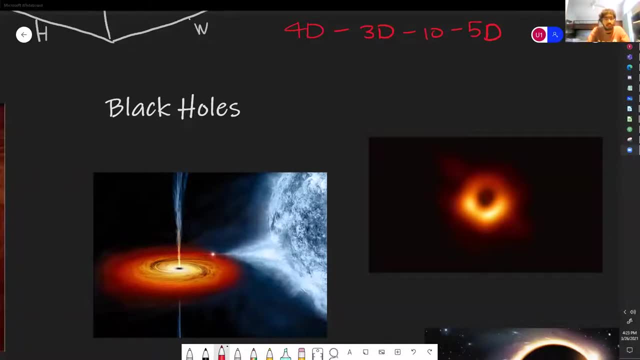 star- yeah, it's a star- more than three times the size of the sun. the, the, the, the, the actual, the actual mass to for a star to turn into a black hole is about 10 times the mass of our sun. oh, whoops, i must have messed up that. so 10 times, yeah, so there's actually a very special. 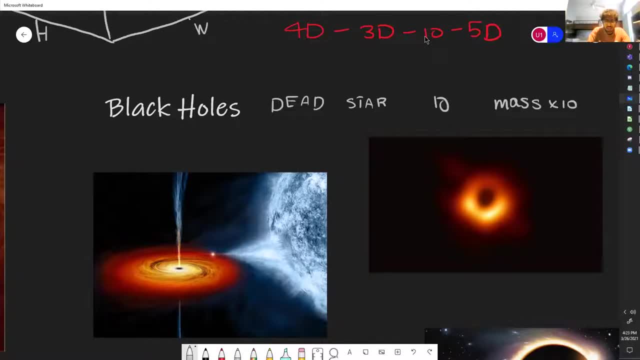 image that i'm glad audubon put on here. so let's look at this image to our right, this really, really blurry looking image. this is a extremely special image. does anyone know what image it is? i think i guess, guys, it doesn't hurt the center of our gallery. 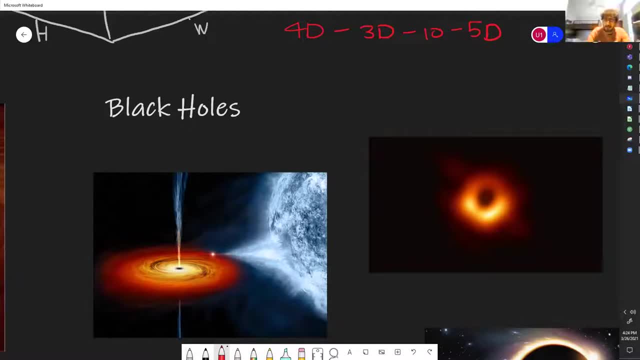 i don't know if it is the center of a galaxy. to be honest, a black hole- yeah, it is a black. this image, the very first image that humans have produced of a real black hole in space, the very first image, and this image came out, i think- i don't know the exact date, but it came. 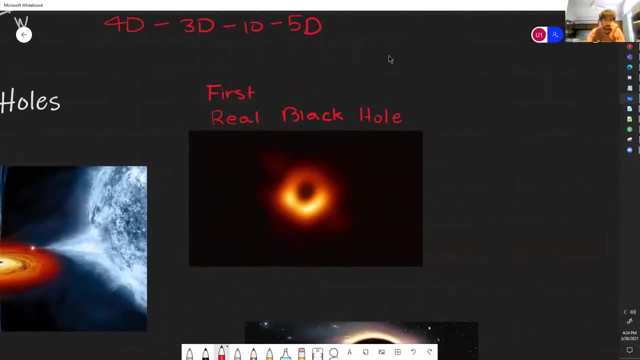 out last year- i think it was in the second half of last year, but i don't know the exact date- but last year we were able to get the very first image of a black hole. so, yay, 2020, something good came out of it. right, that's the only good thing that came out of it. to be honest, that's true, though. 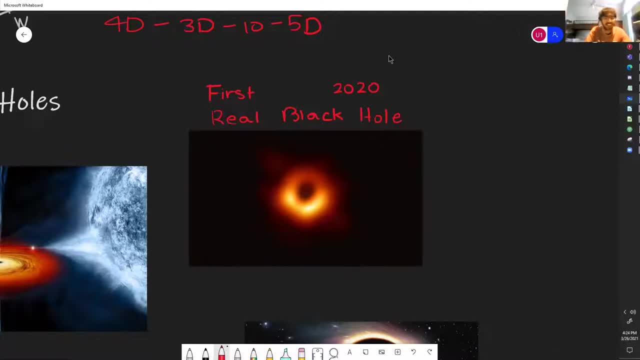 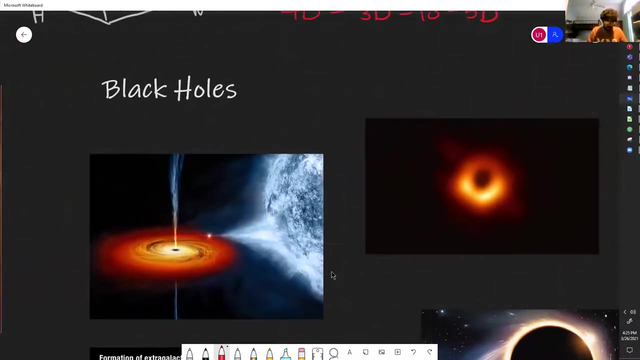 that is true. i don't think it makes up for the year. oh, there are multiple. so before we get into the properties of black holes, let's talk about how they come to be. so, as you guys just mentioned right, black holes come out of stars, and so what happens is that the black holes come out of stars. 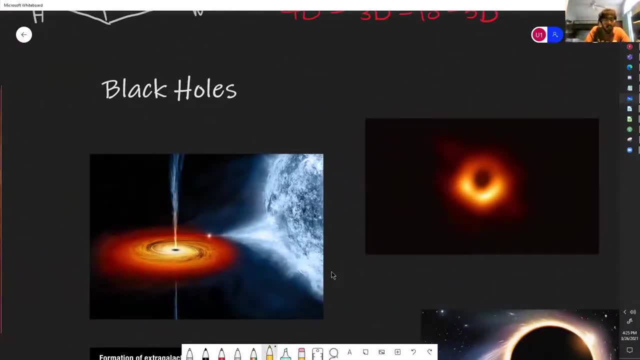 is, stars are originally in in their at the very beginning of their life cycle. they're actually made up of hydrogen, the most common element in the universe, but these stars have to use a process to combine these atoms to make new helium atoms. does anyone know the name of that process? 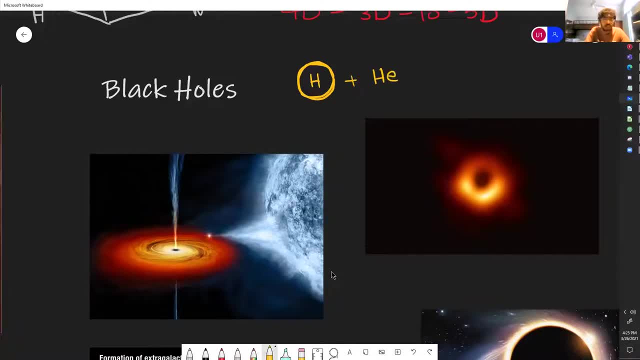 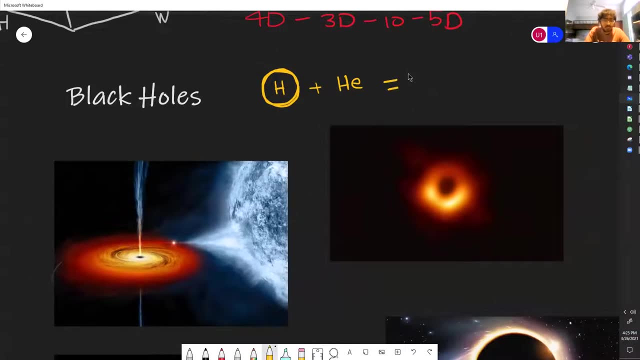 where we combine two atoms to make a new atom fusion fusion. yes, it is nuclear fusion- comes from the center of messier 87, nice, thank you for the information. so, yeah, it comes from the center of what messier 87- yeah, it's a galaxy, it's the super massive. 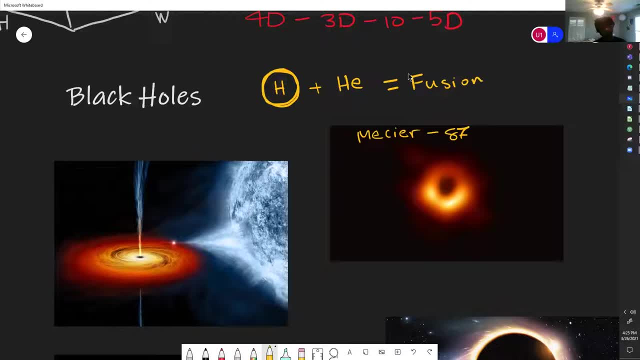 black hole at the center. i don't know exactly where it is. well, thank you for the information, messier 87. that's good to know. josh, you got a question do. has there any of the? is this black part of our galaxy or it's like a whole nother galaxy and it's a completely different galaxy? yeah, how come? 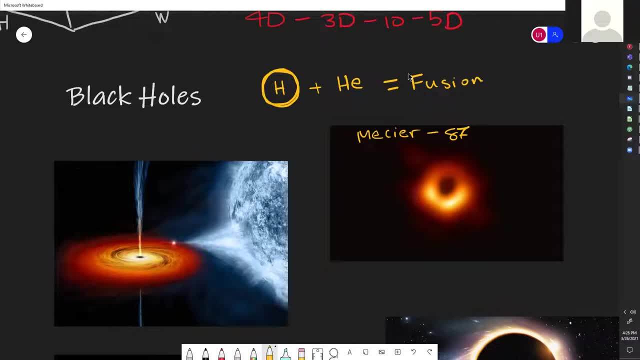 if it's a whole different galaxy, then how? how come we found that first, before finding any black holes in ours? well, we know there is a black hole at the center of the milky way. we do have a super massive black hole at the center of the milky way. however, we are billions upon trillions of 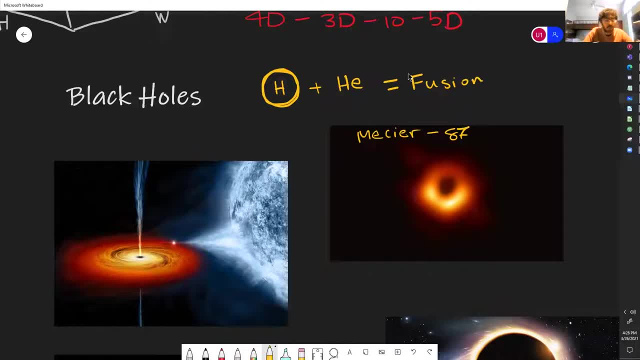 miles away from the center of our galaxy, where the super massive black hole is this. it's in a whole nother galaxy though, so, like this must be the center of the milky way, it could actually be a closer than the center of our galaxy, because our galaxy is really really. 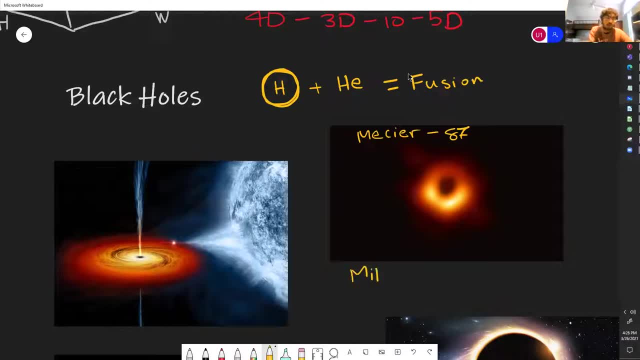 big right. yeah, and also if you want to go directly to the center galaxy from earth, there's going to be thousands of solar systems, thousands of stars in the way that could really pollute the image. they could put like too much light and block out parts of the black hole. so it's really difficult. 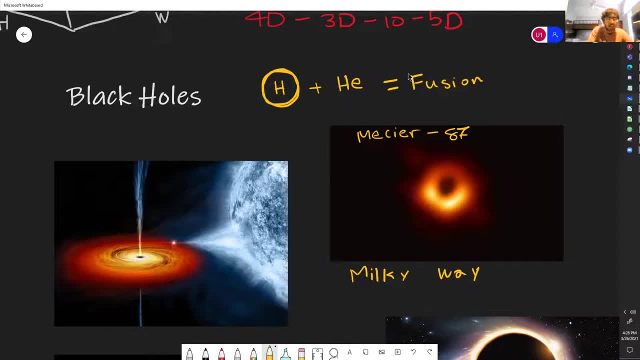 to kind of do that, which is why we try to use another galaxy, because there's not anything in the way except for the easiest example is the black hole, which is the center of the black hole, to explain that: jesh, what's what? wait, which state do you live in? yeah, i see. oh wait, yeah, you live. 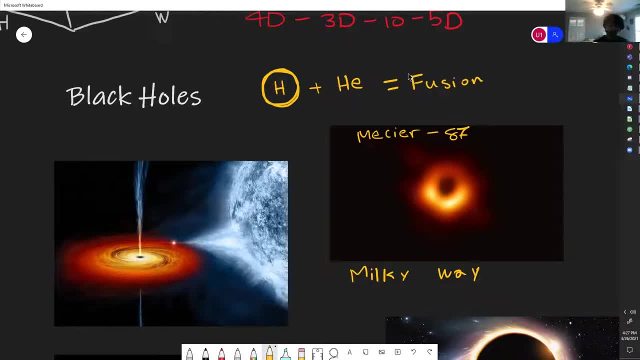 here too, uh well. well, think about it this way, right, would it be closer for us to go? you may think, oh yeah, north america so close, but it it actually may be closer for us to go to, uh, britain than it would be to go to the tip of north america, to the tip of north america, believe it or not. 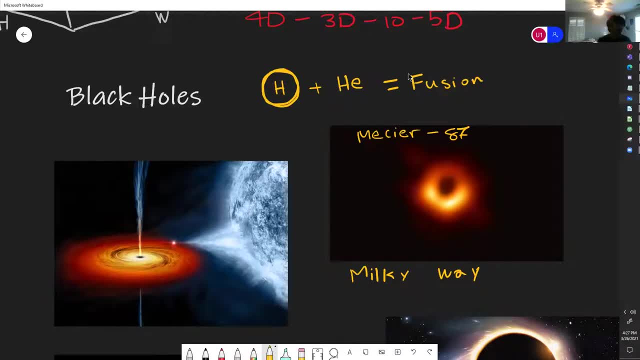 so that kind of explains it right, even though it's completely different parts. it's not even associated with the north american continent. it's closer to go there than, uh, go to the tip of north america. so that kind of so. basically, like there's like. the way that i'm thinking about it is like there's like, like, like. 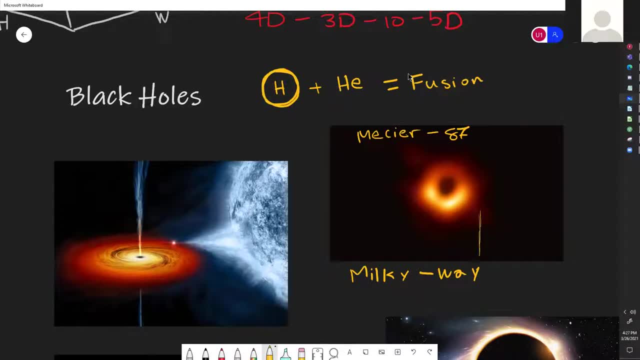 a border around it, like north america, like a whole, like border, like, say, like tennessee, like there's a border for like to know, like which state you're in. is it like that? i guess you could call it that. actually think about it this way, right, if you put a really light, if you put a piece of black paper. 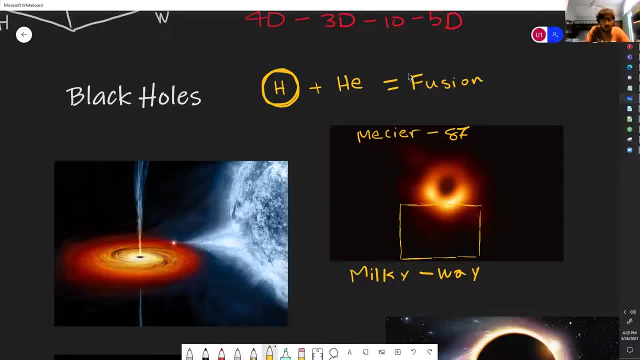 in the center of a room, right, and you put, yes, if you put thousands of candles around it at random locations- right, and you were at the edge of the room. but then there's also black hole that's directly above you, with no candles in the way, which one would be easier to see? 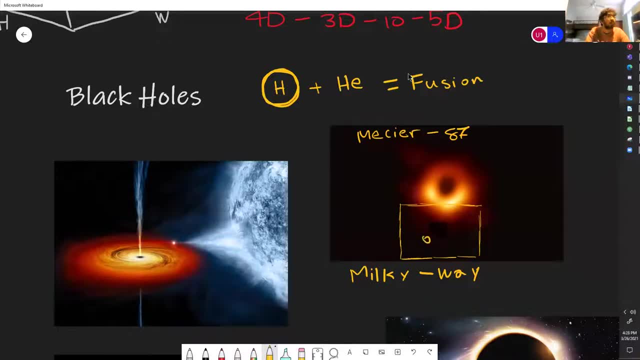 the one above you or the one in the center of the room? oh yeah, that's both of you, because, because all the candles will be blocking the one, exactly right. so the the the black circle in the middle is representative of the supermassive black hole at the center of the milky way. 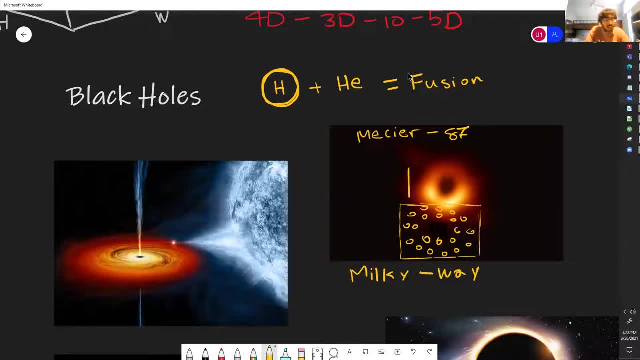 there are millions of stars in the way of earth getting a direct view of the supermassive black hole. so it's easier for us to look outside of our own galaxy and look at a separate galaxy, to look at a completely separate black hole and take an image of that. yeah, we still hope we're. 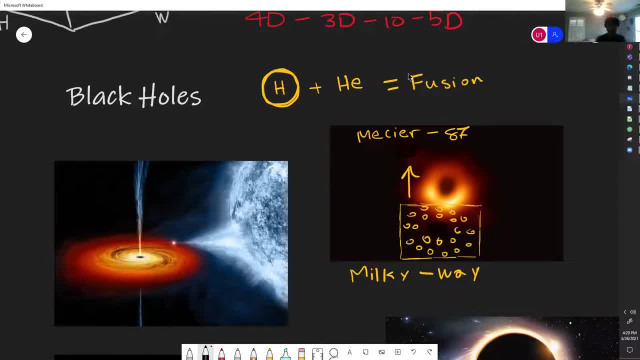 not destroying your minds just yet, but uh, this is at the tip of the, it's almost at the verge. but i think i got it. i have the link for the information page for that specific picture. sure, put it on the chat. uh, let me name. okay, put it on the chat and i will add it somewhere. yeah, so, thank you. yeah so, nuclear. 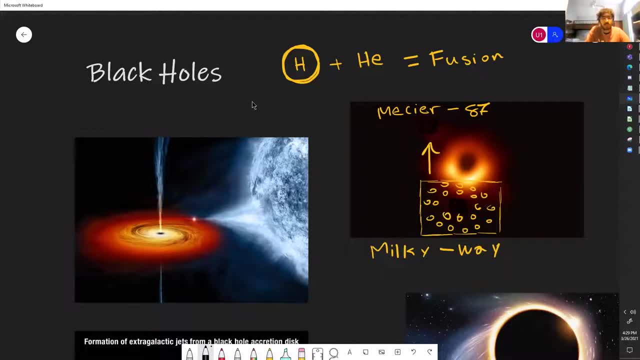 fusion is used to basically make new elements right from height, from uh, hydrogen. so hydrogen is going to fuse into helium and helium is going to fuse into lithium, and all these elements are going to fuse and fuse to make bigger and bigger elements until we reach one very special element, iron. that. 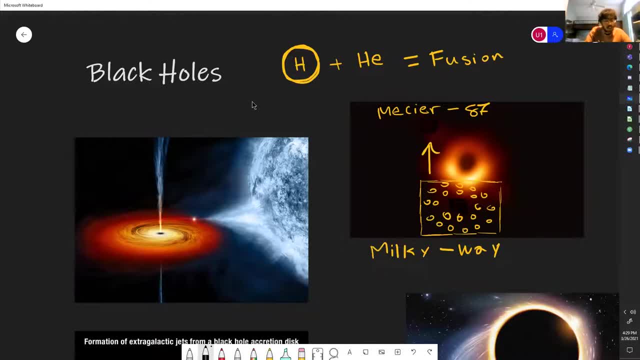 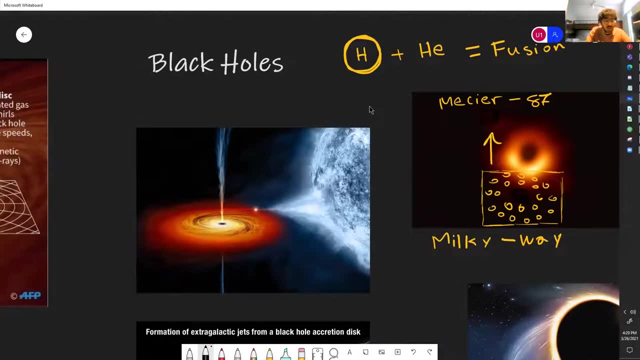 iron, yes, good job. so once this, once the core of the sun, where all this nuclear fusion is taking place. once the core of the sun begins to make iron it, it can't use the iron anymore, because the iron is simply too heavy. it requires a lot of energy to fuse into helium. so it's going to 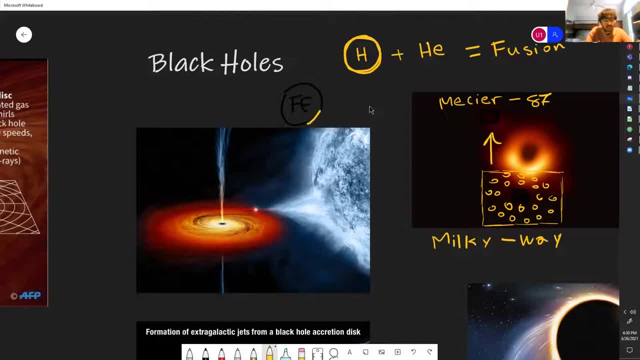 require too much energy to fuse into a heavier element than it makes. what a fusing iron uses more energy than it makes. exactly right, the sun would be wasting energy. it wouldn't be able to do it, but the energy it has. so the iron is simply going to build up in the core and this is what happens. 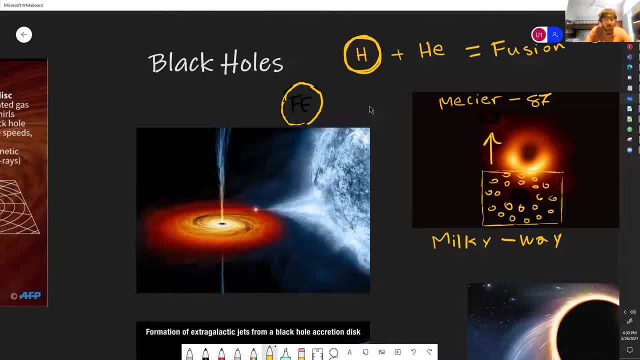 when you reach the end of the life cycle of the star right, because it's basically almost run out of fuel. when once it's made iron, because from now on every time it fuses it's getting closer and dying because it can't fuse iron anymore and so eventually the force of gravity from these iron 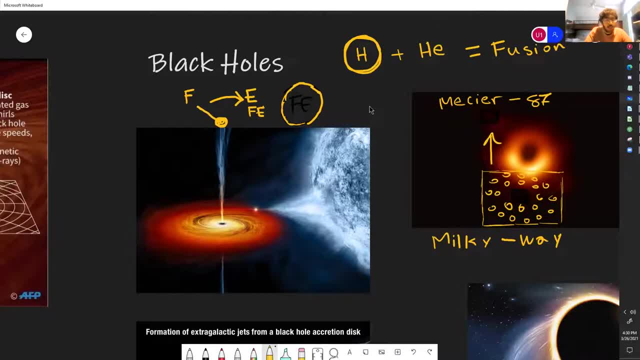 particles in the sun's core is going to overpower the nuclear force that's keeping all these ions and atoms close together so that they can fuse and, as a result, the sun is going to implode, it's going to collapse upon itself and when it does this, it creates this kind of explosion. does anyone? 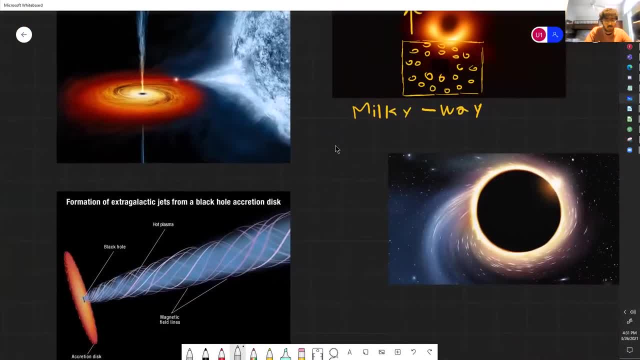 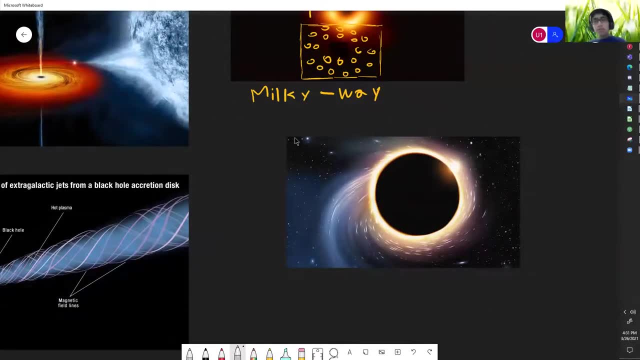 know what that explosion is called supernova, but i think that the sun is too small to make a supernova. the sun is too small to make a supernova. yes, it is so. yeah, so this, the star, is actually going to make a supernova. it's going to collapse upon itself and then explode outwards, leaving 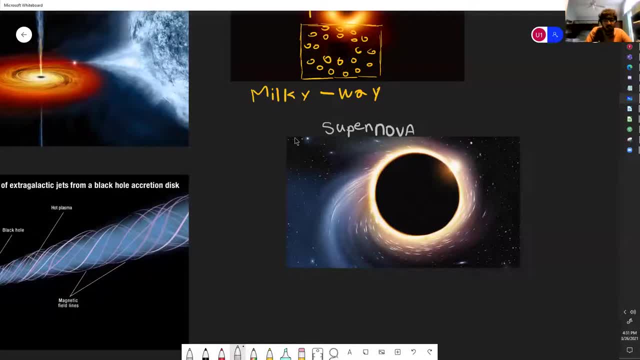 behind one of two things: if it's not a, if it's not a very, very, very big star, it can leave behind a neutron star which is like a super bright white star. or if it's more than 10 times the mass of our sun, then it's going to implode into a black hole. 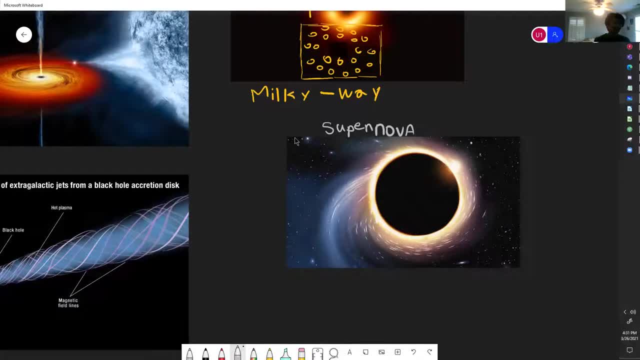 okay, so any questions about how black holes are created? small anecdote guys, you see how, uh, well, this is an interesting thing to say. oh, reika, do you have a question? actually, i know another way you could create a black hole. okay, you just have to say, you just. 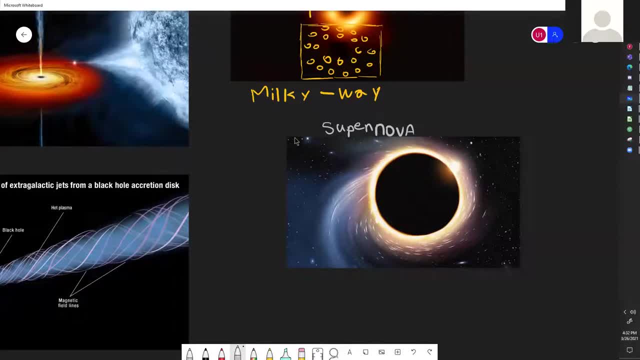 have to shout something out louder than 1100 decibels. oh great, i've heard something along those lines. yeah, i wish you luck doing that at 1100 decibels, but you see something like that and your voice is gone for the rest of your life. uh, i don't think it's, just your voice is off. i. 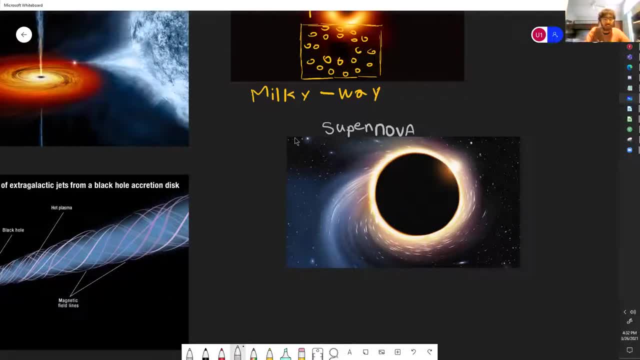 bigger problems are away. i think you'd be killing it like people within earshot. but uh, you see something, guys, uh, to notice with this. a small anecdote is: you see how arav knows a bunch of this stuff? interestingly, i'm learning half of this stuff for the first time. 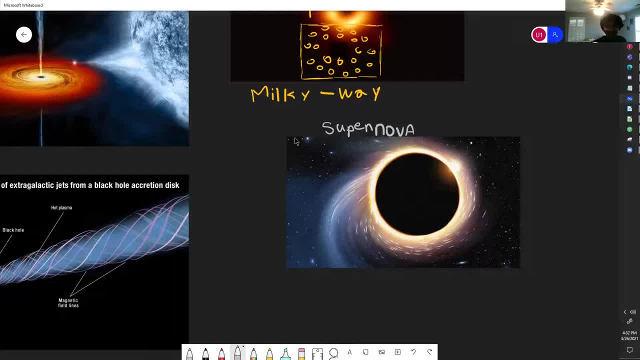 so you see, age and science doesn't matter. it's, it's all relative. i am not at all any bit experienced in this and i'm not going to be able to do anything about it. i'm going to be able to do anything about it and therefore that shows why, you guys, we all have our strengths. we all have. 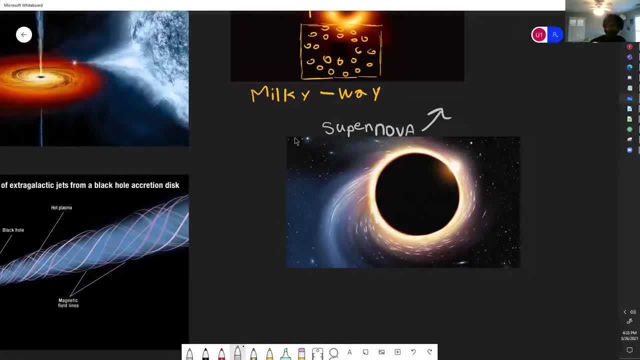 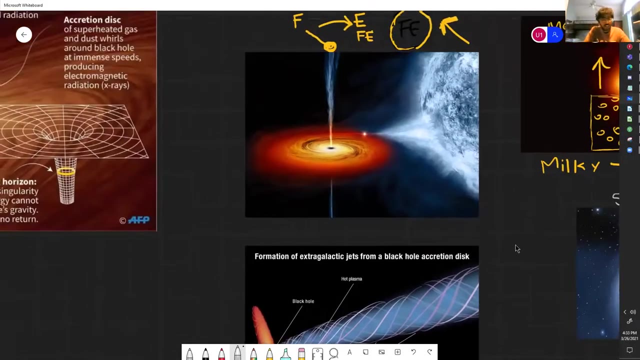 our weaknesses, exactly right. and it doesn't matter how old you are. you can be with and you can know something much better than someone much older than i. mean, that's a good anecdote for why we do this. yeah, so when continuing in the lifestyle life cycle of a black hole, right, this is only the. 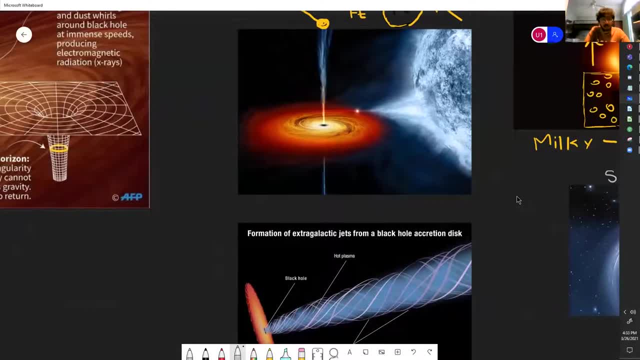 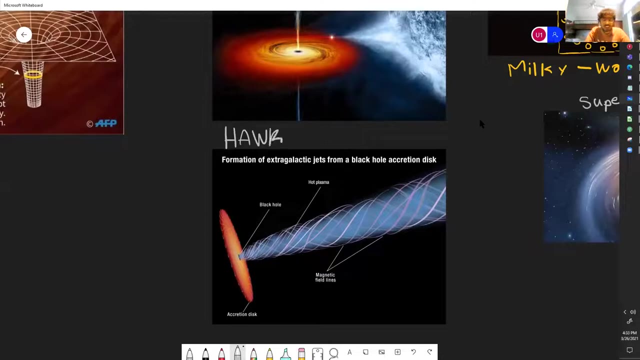 birth. so this black hole is slowly going to evaporate, which we will talk about how it does shortly, but it will evaporate. that and after hawking radiation, hawking radiation- we will talk about hawking radiation. so after about 10 to the 54th years it will disappear. and since we probably 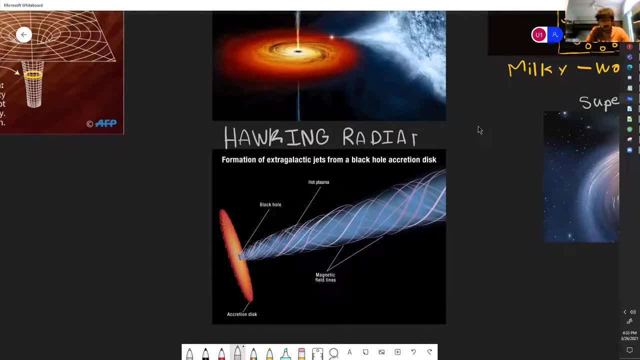 won't be around to witness one. we don't know what's going to happen. scientists have no clue what happens when a star dies or when a black hole dies, so that's something we'll have to wait and see. hopefully it doesn't. hopefully we're around by then. okay, so that's it for the life cycle of black. 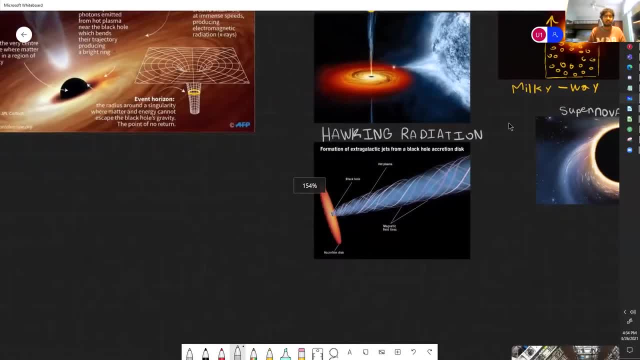 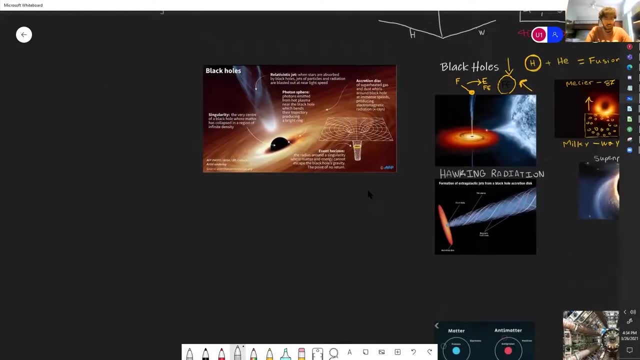 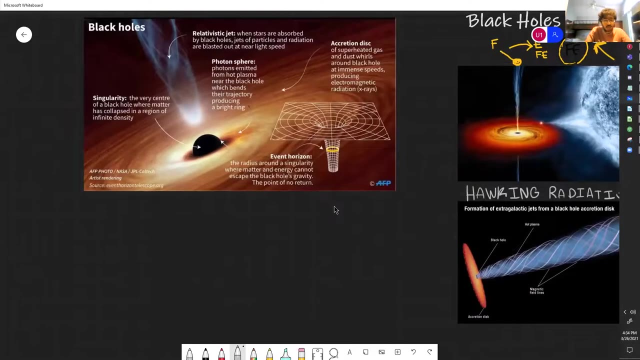 hole. it's born from a star. it slowly evaporates and then disappears through something that no one knows about. so now let's talk about the structure, or like parts, of a black hole. okay, so what? when you guys think of black holes, what do you imagine in your head? what, what do you see? 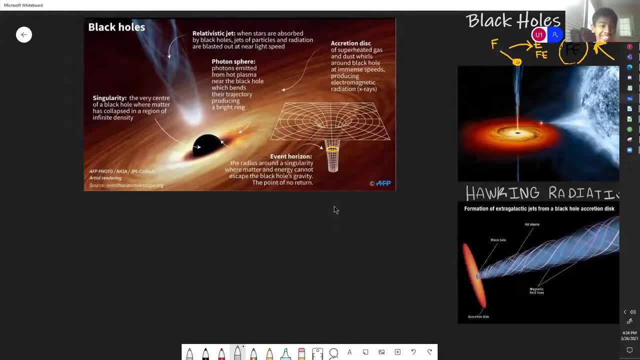 like an invisible circle or an invisible tornado in the space, okay, anything else, uh like, uh, like a comet trying to go through something. okay, i don't know about you, shimon, but when i see a black hole, i just think of bubble tea, pearls. you know, that's a very accurate representation. 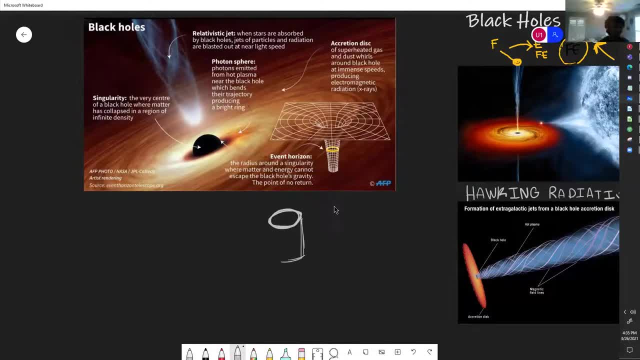 anymore. you guys, do you guys think of bubble tea pearls when you're in a black hole? you guys, do you guys think of bubble tea pearls when you're in a black hole? when you're in a black hole like bubble tea, have you ever tried it? let me drink your coffee. no, it isn't like real tea, guys. 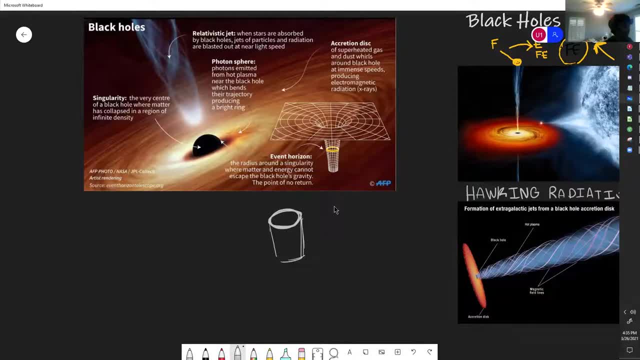 it's, it's a delicious thing. it's like. it's like this nice milk, uh, like milky, milky, like fruit flavored drink with, uh, these pearls on the very bottom that are made of tapioca, that are super. you should try it. sometimes bubble tea is pretty good, it is very good every like. so, yeah, well, when. 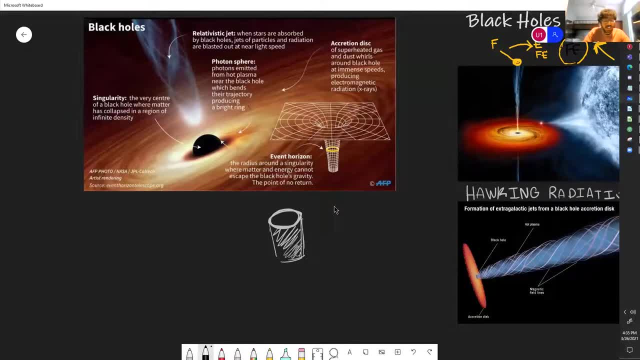 we look at black holes in space, right, we can't actually see them because they're black and space is black. oh wait, wait, before before that. what is? what's your question, sandy? please tell us. i was gonna give another description of a black hole. i think it's like, kind of like. 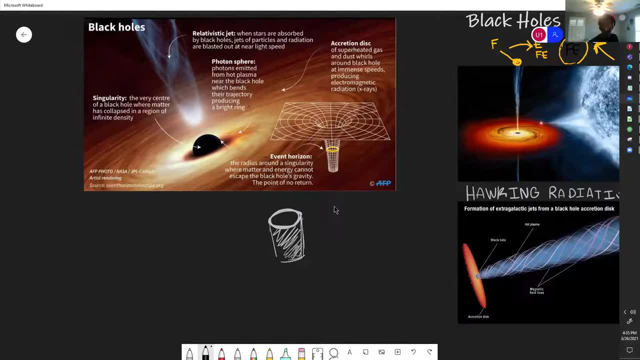 oh, oh wait, kind of like some trap which sucks things up and and never lets them go. mm-hmm. yeah, what about you, sandy, please, uh, please, tell us. uh, you never knew. um. so i had a question. um, if scientists have like never seen a black hole die or anything, how do they know what actually? 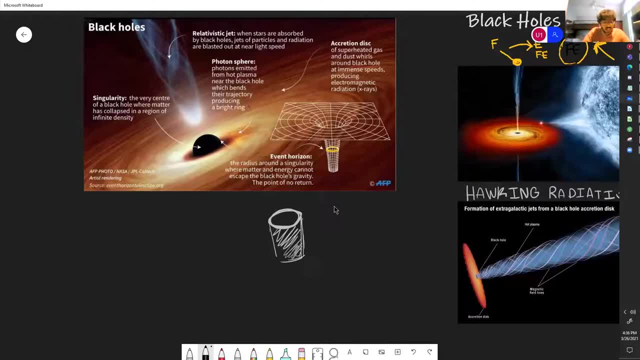 happens. see, they didn't actually until a couple years ago. so there's a scientist named stephen hawking who actually came up with the theory that black holes emit these particles. that slowly makes black holes shrink and shrink, and this theory was never actually proven until, i think, like nearly. 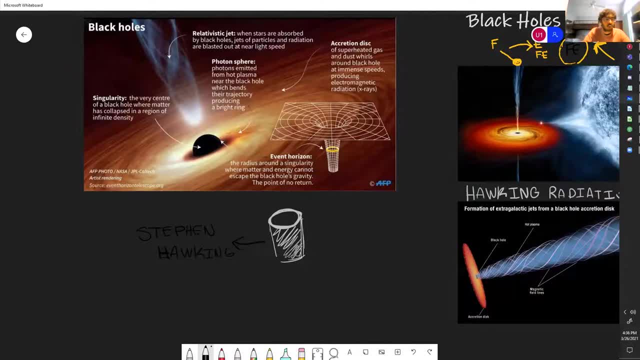 seven-ish years ago, when two black holes uh combined to form a supermassive black holes, scientists were able to detect traces of the radiation that is being emitted by the black holes. so they didn't even know that black holes could die until very recently. okay, thank you. yep, uh, don't get scared, but that is uh, stephen hawking. 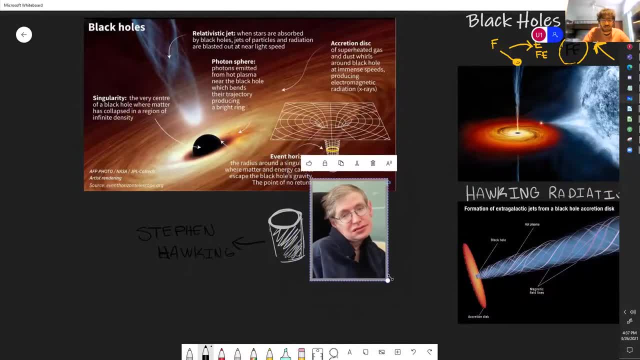 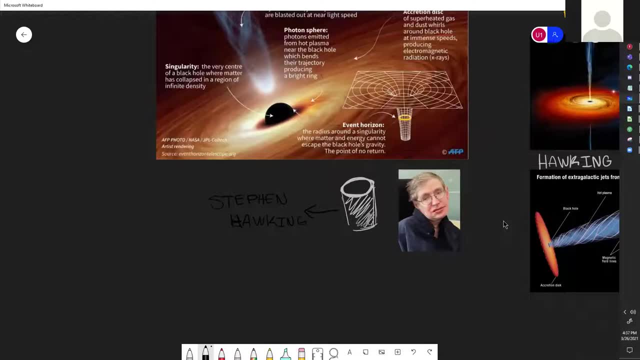 and he died very recently, which is a true shame, not very, very, very a couple of couple of years ago. there's a movie about him. what happened to his neck? well, he had a disease where he he couldn't like move around a lot. yeah, he suffers from a disease called a als or lou gehrig's disease, and 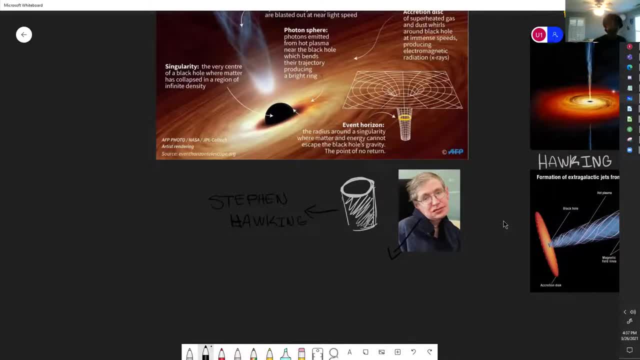 what happens is that over time, all your muscles paralyze and you can barely do anything. and this guy, by the end of his time, the only thing that he can do is he can't do anything. and he can't do anything because his only muscle that was working was a cheekbone, and to speak he would have a. 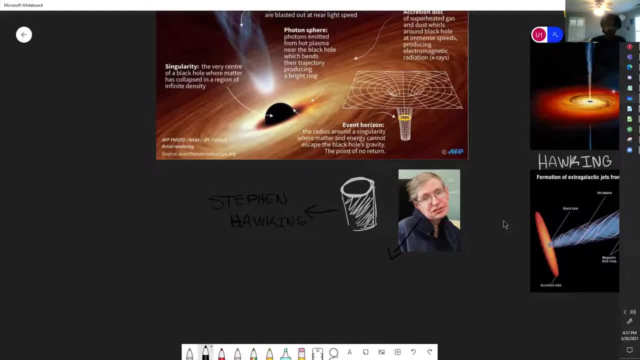 button that he could, that he can right next to his cheekbone, which he could like press by, like manipulating his cheekbone a little bit, you know. and he spoke by like literally using that button and kind of doing like some worst code language and he did lectures with that. can you imagine? 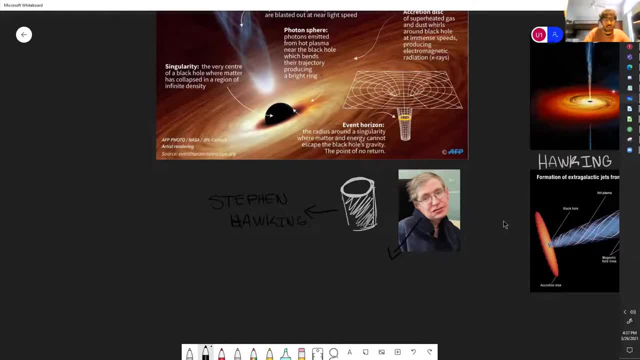 did make a very special computer that basically said what he was trying to say. this button, yeah, but he did. he lectured with this much difficulty, which is amazing. the tenacity, the, the, the heart of the, is really amazing. you guys should definitely learn about Stephen Hawking. 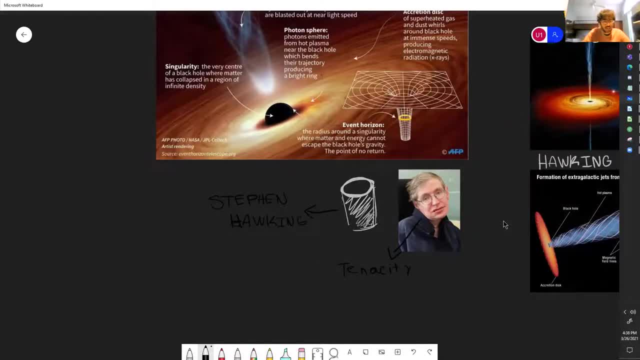 he does have a couple shows. I think there's like a couple on Netflix. you can find plenty on YouTube. he did have some really really interesting shows about time and space in general, so I would very I would recommend checking those out. they're really really interesting. his mind was running. 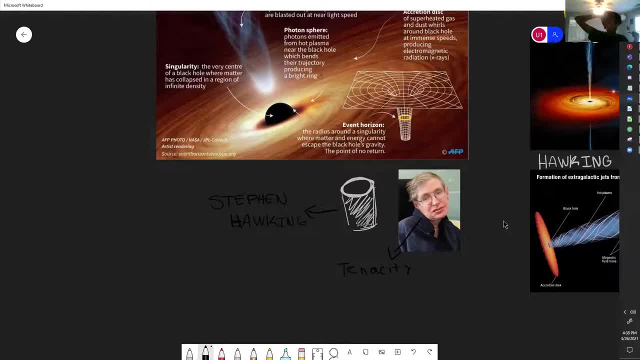 around the universe, even though he was in one place, yep, yeah, and also back to the parts of a black hole. oh, one, one more thing. and also, if you're just joining Tavish or Samyuka, yeah, you were probably very lost, but wait till the end. we can, uh, go over what you did miss and today's 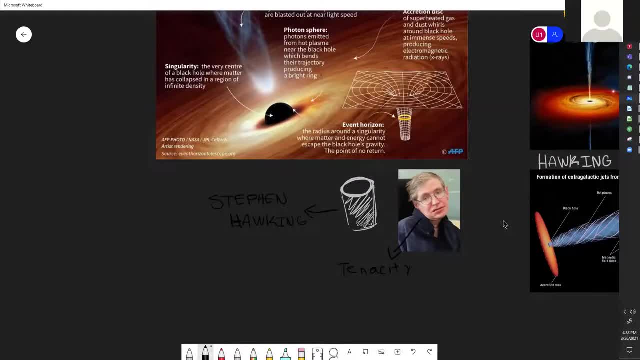 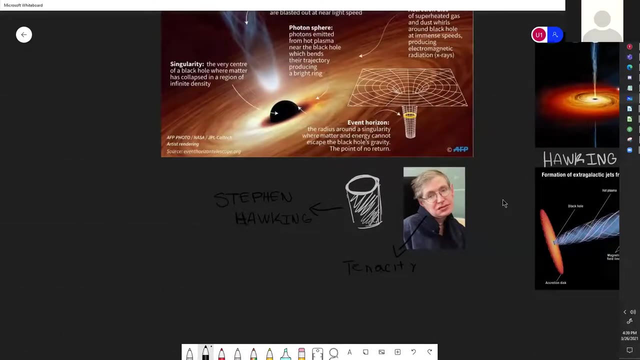 really just a fun entertainment lesson. I was gonna ask once class was done. yeah, yeah, today's a very chill, entertaining lesson that you're gonna And it's just relaxed, It's not that hard. Are we going to do quizzes? Yes, we will be doing quizzes. 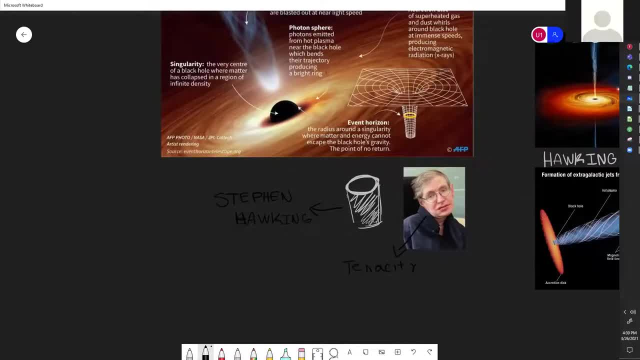 Whenever I hear black holes, I know they're not quicksand, but they remind me of quicksand. You know, I also think of that, And that's a very good observation. So let's look at the parts of a black hole. 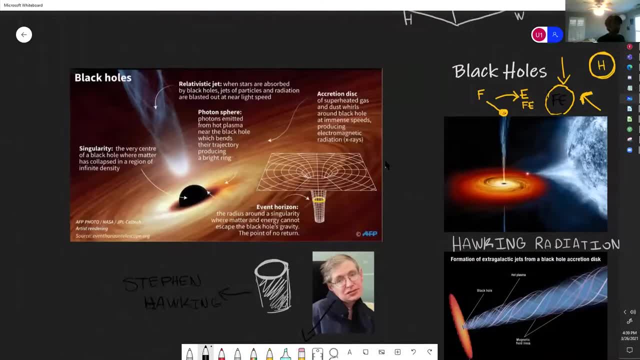 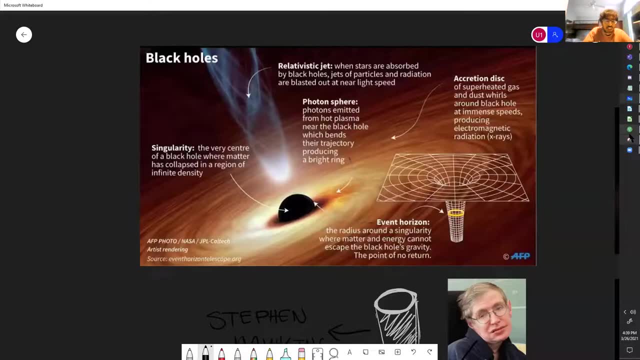 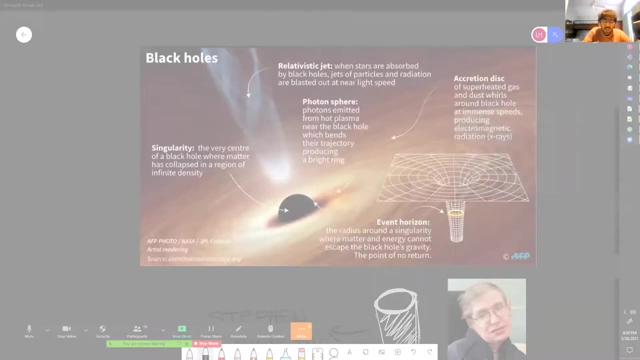 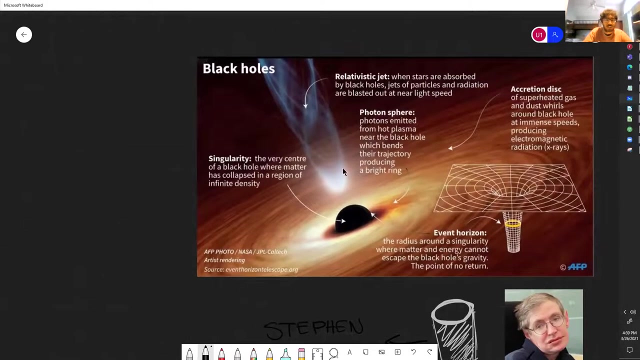 We're starting to be a little late. Yeah, So there are a couple of parts to a black hole, right. So the part at the very center, the heart of the black hole, is what we call a singularity. So a singularity is basically a single point of very, very small area in which an incredible mass of a star is concentrated. 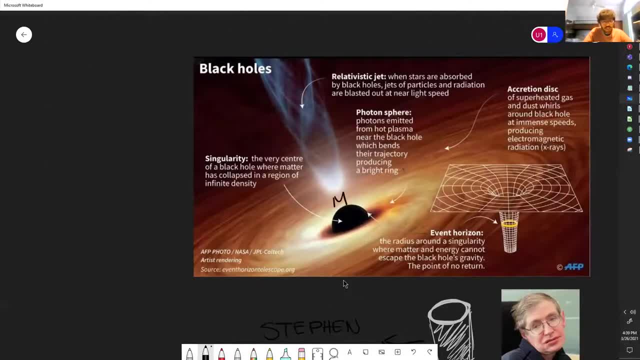 So, for example, for us to have a black hole right, we would have to take our entire sun in all its mass, And we would have to concentrate. We would have to concentrate it down to the size of New York State, right to the size of one state on Earth. 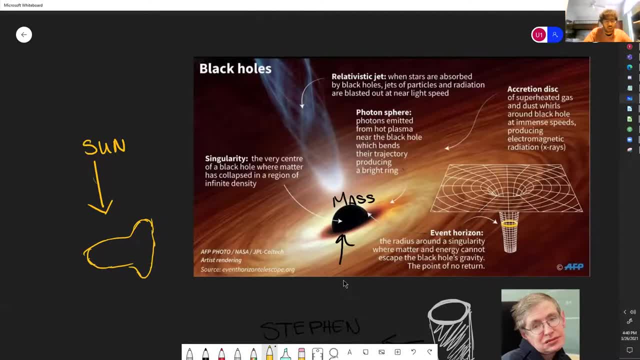 And for comparison, I think it's around like 1,200 Earths can fit into the sun, So we would have to take the sun and fit it into this really, really small area right, And so this creates an incredibly strong gravitational field because it warps the space-time fabric by a lot. 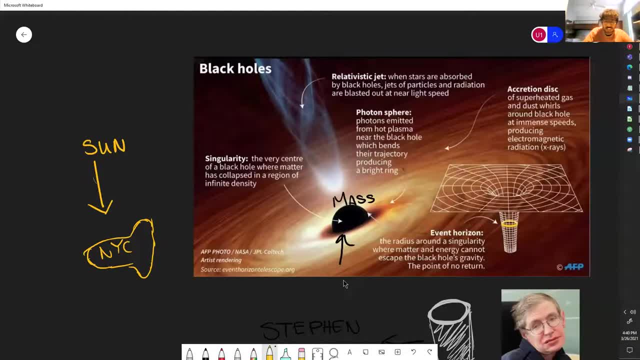 So if you look at this diagram of, like the space-time, it's like a well right, It just like goes straight down And that really shows the steeper it is, the stronger the force of gravity. So this is super, super steep. 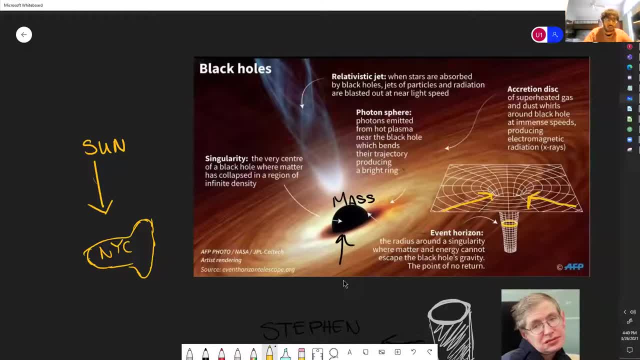 And so it has an incredibly powerful, really strong force of gravity. Yep, That's at the heart, And then around the heart we have what we call the event horizon. The event horizon is the distance at which anything inside the event horizon, nothing, can escape. 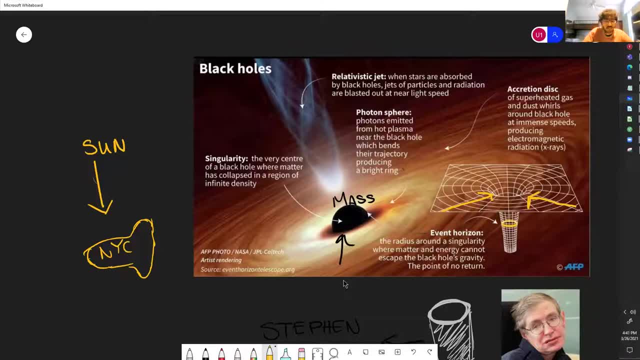 Not even light can escape once it's inside the event horizon. So it's like that keep-out sign: If you cross, you're dead. What's your question, Sunmiq? So technically that space, that gravity becomes more when you go closer to the middle. 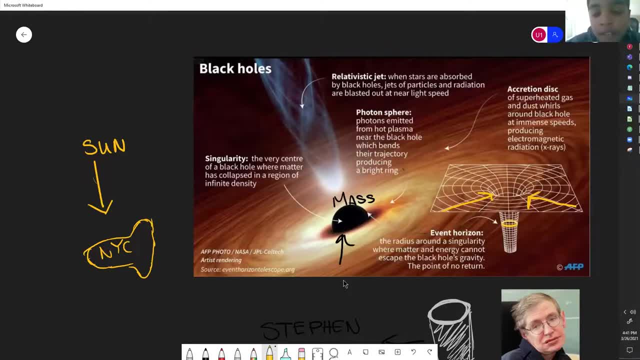 I feel like it's kind of like it wants to take the thing. The more you go inside, the more you pull it, The more it pulls. Like I've been reading this book on five kingdoms and they kind of talk about they have something called. 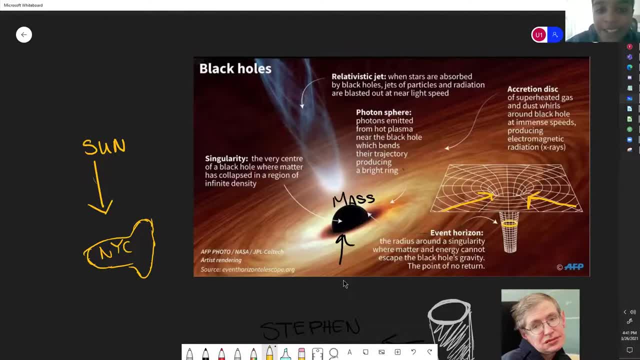 they have a land called the land of the dead or something, And when you go to the echo lands- it kind of it's called- becomes stronger. So technically, if you think of it like that, it kind of makes more sense that the more that you go closer to the inner part, 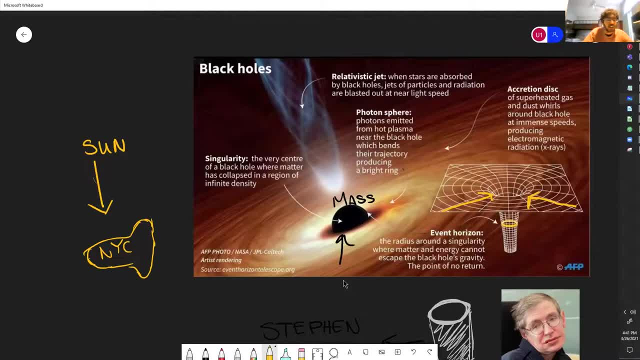 the gravity becomes stronger. Yeah, It's kind of like trying to dig out a hole right, Like the deeper you get into the hole, the harder it is to pull yourself out of it. Oh yeah, And once you cross the event horizon, well, good luck. 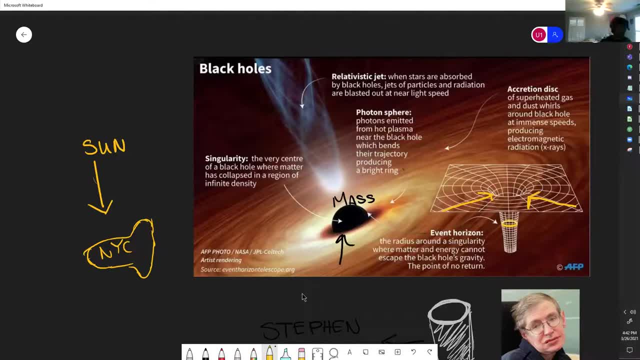 You can't get out. Yeah, One more question. Yeah, Sunmiq, do you have another question? No, I'm sorry, I forgot to put my hand down. Oh okay, My bad, Okay, Okay. So around this, around the event horizon, we have what we call the photon sphere. 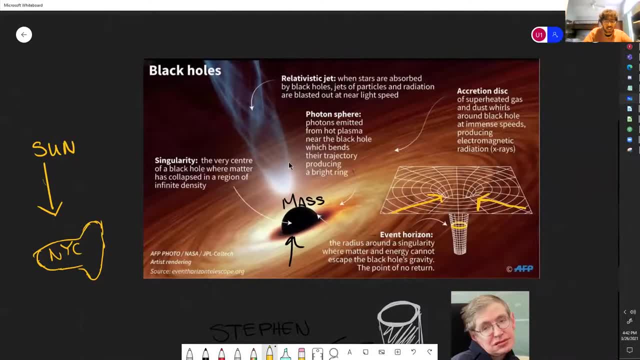 So the photon, The photon sphere, is basically like it's like a cloud of light. It's where all the photons are being bent by the force of gravity but they're not sucked in because they're outside of the event horizon. Okay, 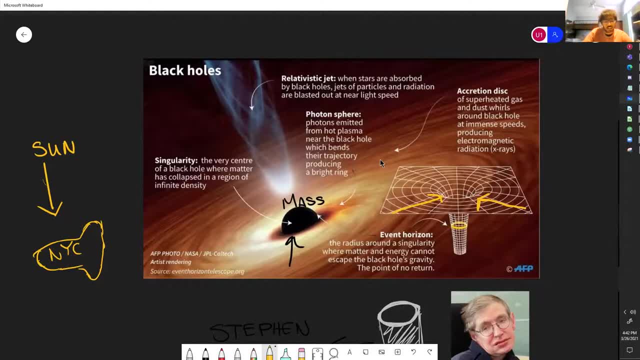 There's also something called the accretion disk. So the accretion disk is basically a disk of plasma, which is the fourth state of matter. It's made up of a bunch of supercharged ions, So this disk just revolves around. 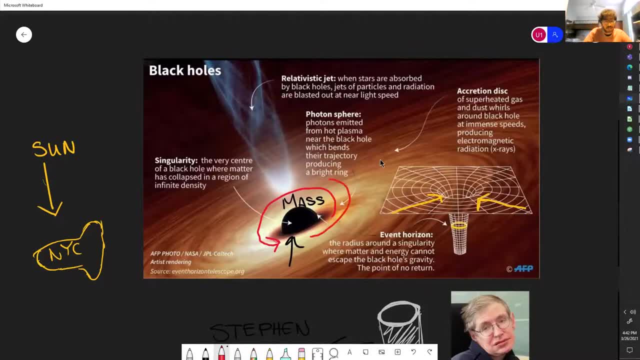 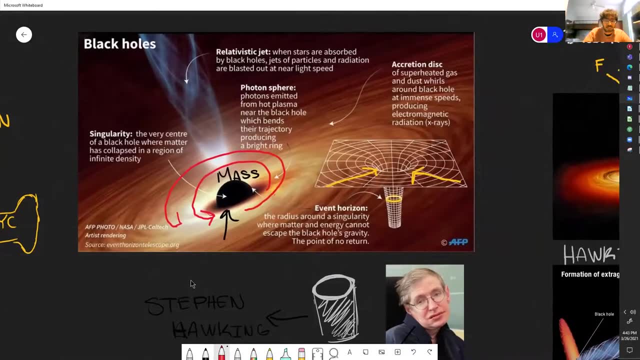 A black hole and it can be drawn from stars. So when a black hole eats stars, right, Not all of it is going to go inside the black hole. Some of it will condense to form this accretion disk. And then we also have the relativistic jet. 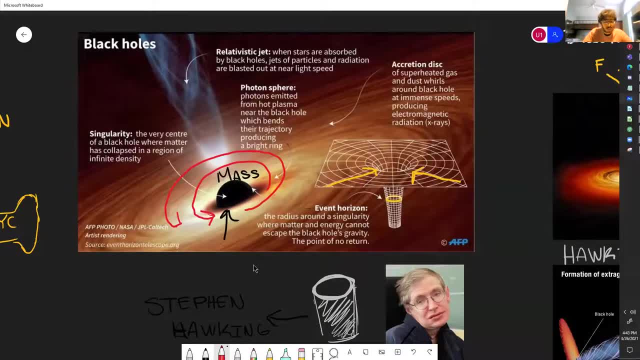 So some of the plasma is not going to go to the accretion disk. It's going to be ejected by the force of gravity outside. So the reason why it is ejected is because it's spinning so fast around this black hole that it 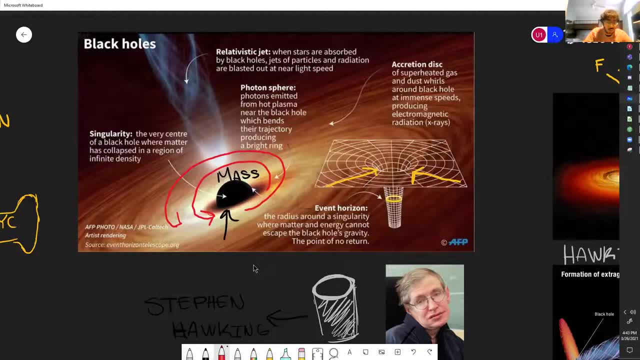 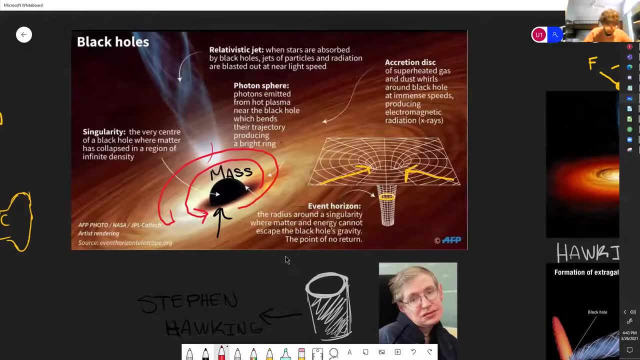 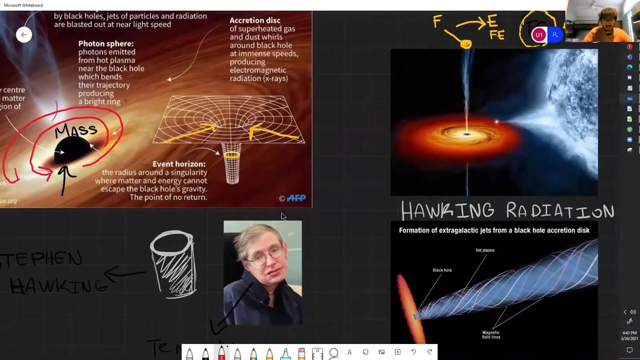 Begins to go around and below it and then eventually, it's just going to be pushed up by its speed. that's pushed away by its speed, Okay. So any questions about black holes? No, Okay, Then we have one last thing to talk about: black holes. 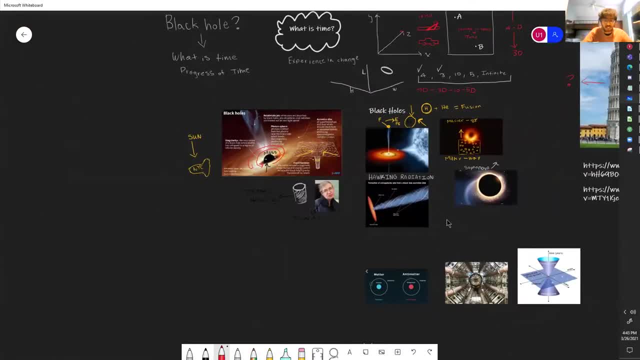 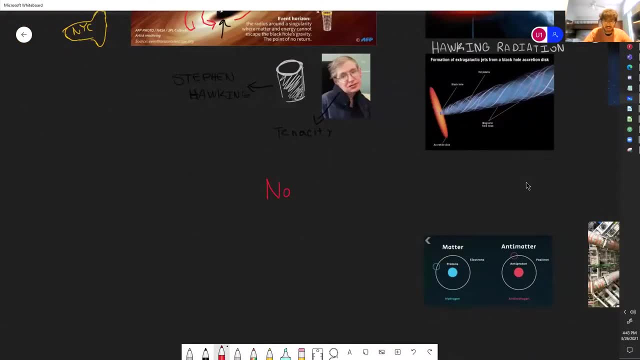 So the last thing I want to talk about is what is called the no hair theorem. So the no hair theorem is something really simple, right? All of the no hair theorem says Is that there are three factors that differentiate all black holes. They are mass charge and angular momentum, right? 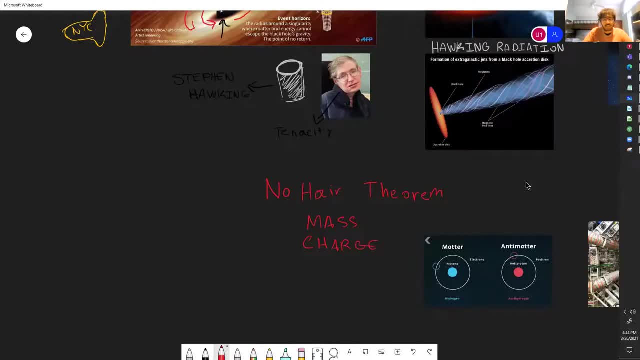 So the mass is basically like: how much stuff is there? The charge is: well, you know how positive or how negative is it? And the angular momentum is basically really: how fast is it spinning? Okay, That's angular momentum is just looking at how fast it is spinning. 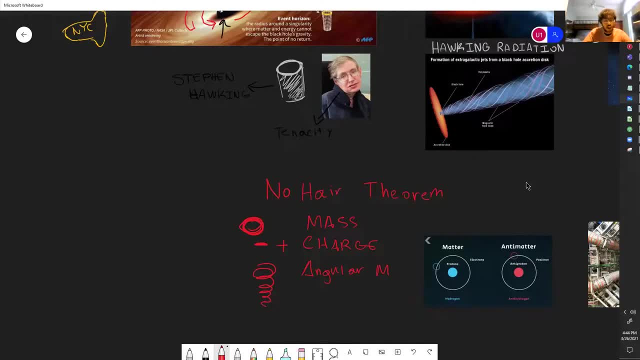 Okay, So all the no hair theorem says that all black holes differ in at least one aspect. So, for example, if you had a black hole with the exact same mass charge and angular momentum, you're talking about the same black hole, because there can't be another black hole like this one. 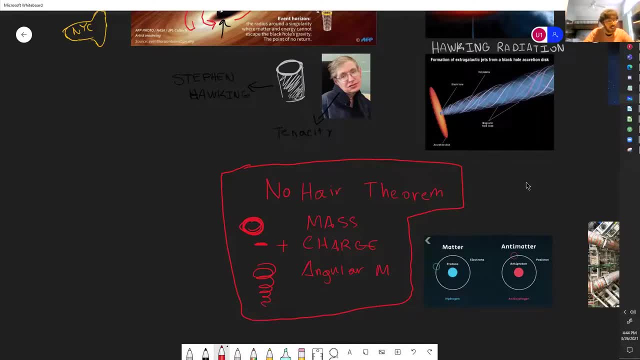 It would be an exact replica of the black hole, but you can have black holes with, for example, the same mass, the same charge, but a different angular momentum, or maybe the same angular momentum. Okay, So they have to differ in at least one of these three aspects. 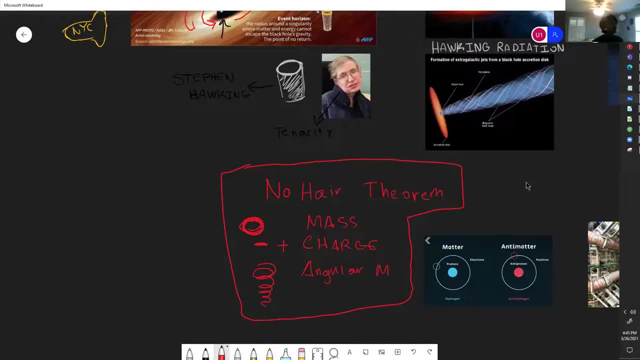 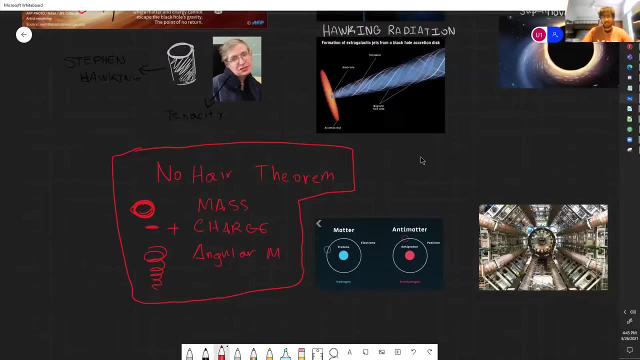 Yeah, And that's all it really says. And, if you like, you don't need to overthink this. Just think of the no hair theorem. mass charge, angular momentum, Yep, How exactly does Hawking radiation work? again, We're about to talk about that. 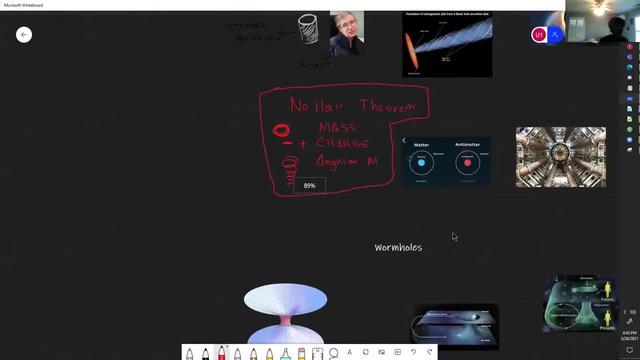 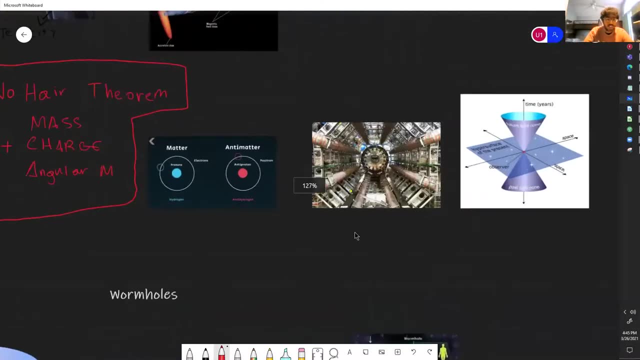 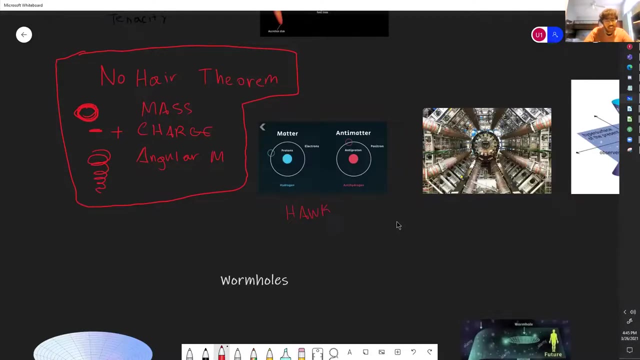 So in Hawking radiation, oh, we're really running behind. So in Hawking radiation, what's actually happening is You have a particle-antiparticle pair that's going to pop up So across all of space. right, You're going to have these antiparticle and particle pairs that are going to be made due to quantum fluctuations. 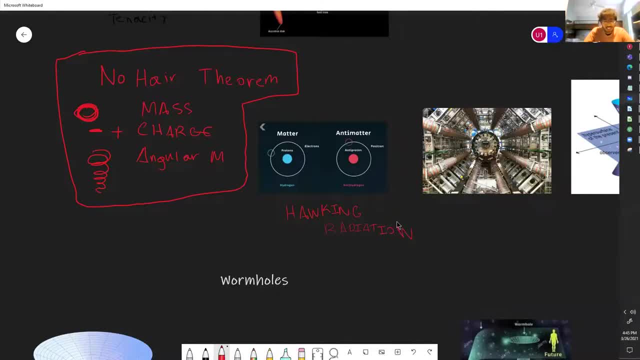 And then, once they're made, like literally the next instant, like almost instantly, they're going to combine and then turn into pure energy and then return to what they came from, Right, Because, if you remember, Mass is energy, right. So the energy is going to condense into mass, into antiparticle and particle. then they annihilate each other and turn back into energy. 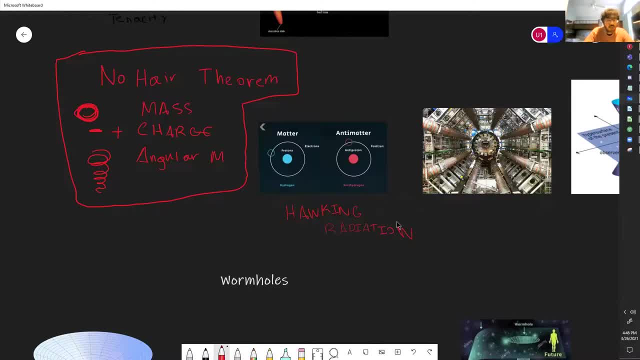 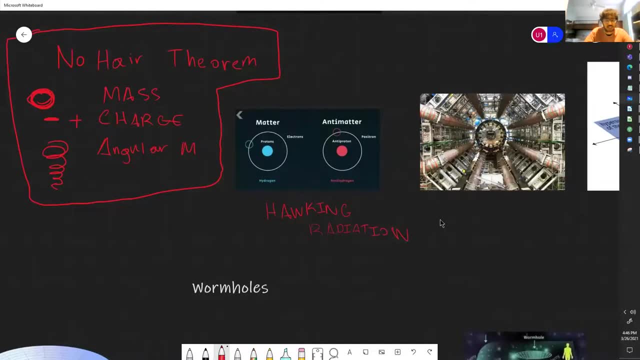 But when you go near a black hole, sometimes these pairs are going to form on opposite sides of the event horizon. So you're going to have one particle inside the event horizon and one particle outside of the event horizon. Yeah, So in order for Hawking radiation to work, 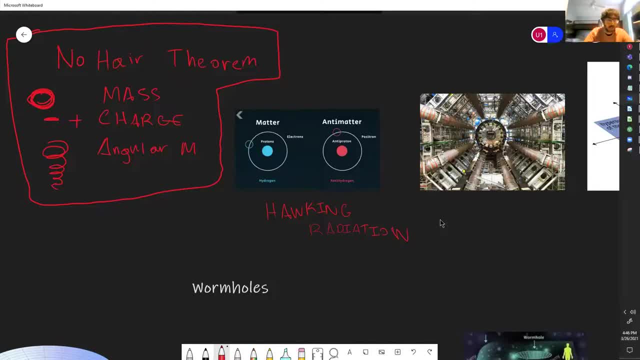 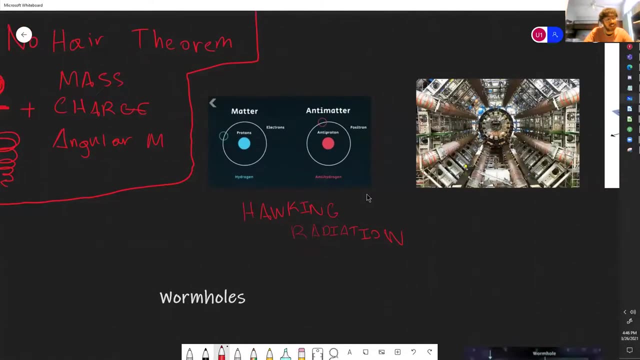 You need the regular matter particle on the outside and the antimatter on the inside. So the regular matter particle is going to run away from the black hole because it doesn't want to be sucked in And the antimatter is doomed because it's stuck inside the event horizon and nothing can escape. 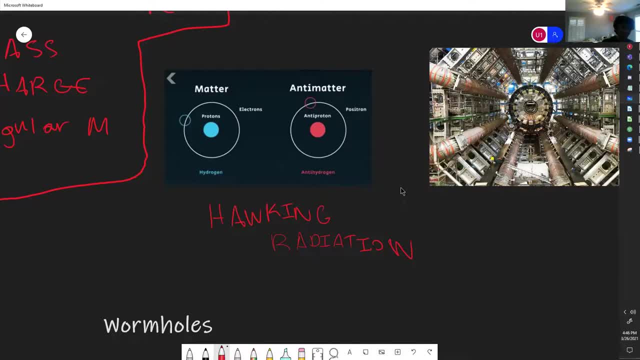 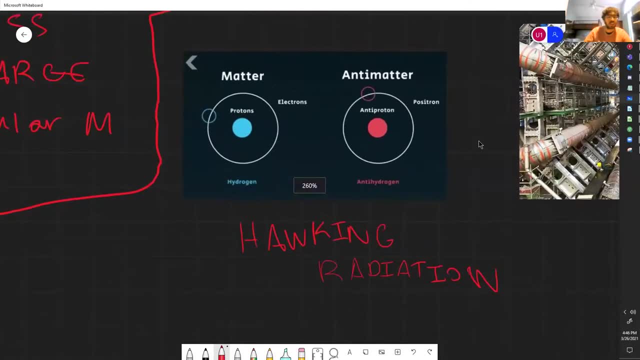 Yeah, even I'm getting confused guys, So don't worry about it. Yeah, I don't think we'll be able to cover everything that I had planned for today, So I will make a video of everything we didn't get to talk about. 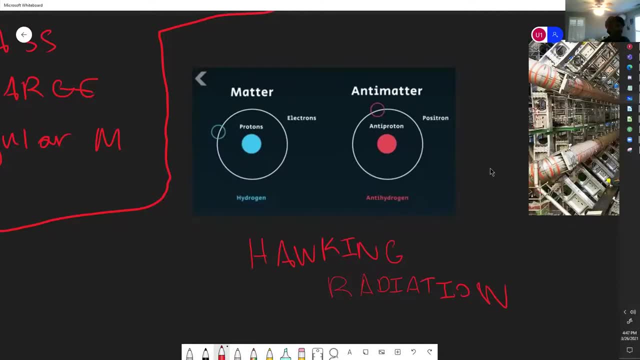 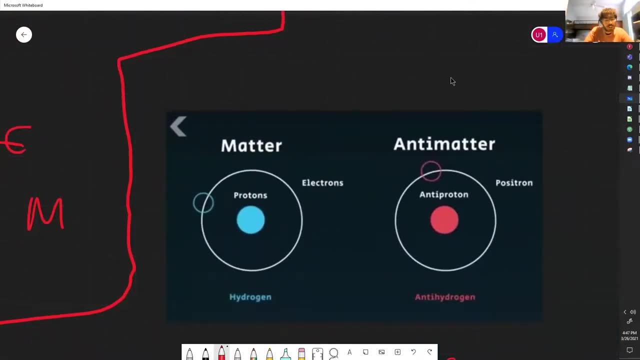 Well, we still have a couple of minutes so we can still go over some things. Yeah, We still have time to go over stuff. So this antimatter, really it's the opposite of regular matter. You can think of it as negative mass. 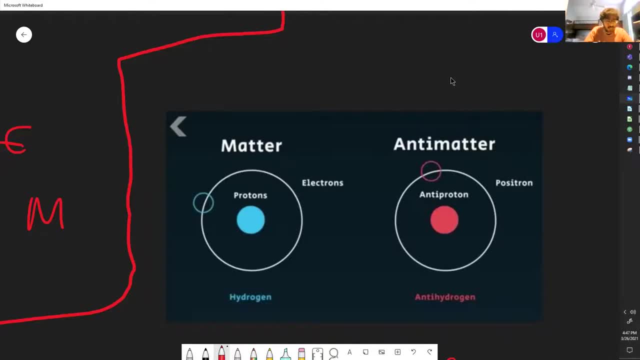 That's a really weird concept, right, Negative mass, But that's what you kind of have to think of it as. So If the antimatter goes toward the singularity, it's actually going to cause some of the mass of the singularity to disappear. 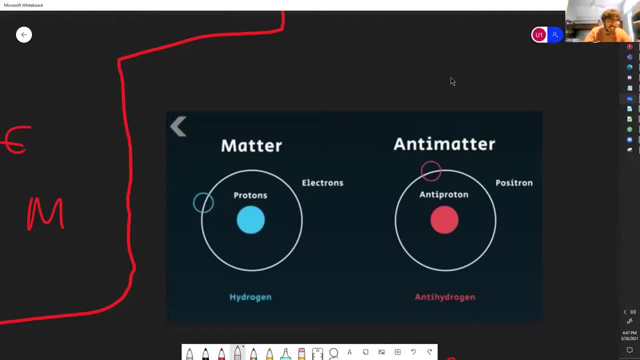 It's going to annihilate some of a tiny, tiny piece of that mass, And so the black hole slowly loses energy over a gigantically large period of time, right 10 to the 54th years. Okay, So with antimatter at least, let's not worry about that. 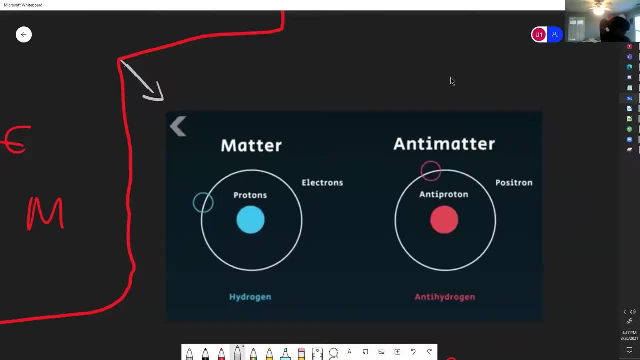 Let's just go over the basic differences at this point on antimatter. So Yeah, I'll go over it because I feel absolutely useless. But it's okay, I have to feel useless once in a while. So what do you guys? simple review. 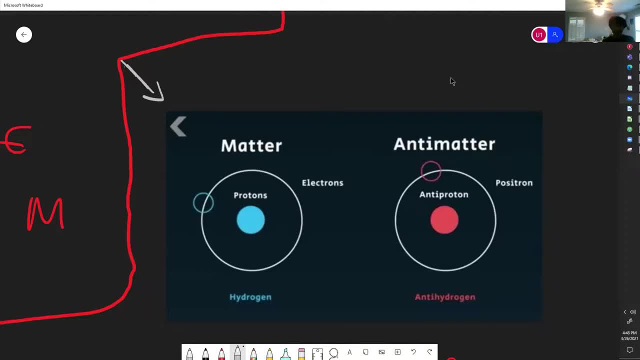 What is the charge of an electron Minus two? Wait, what Negative, Yep, yep. What is the charge of a proton Positive, Positive? What is the charge of a neutron Neutral, Zero, Neutral, Good. 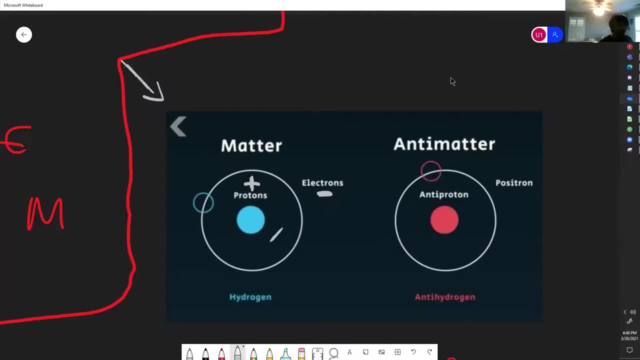 Now, antimatter is just the opposite. What do you think the charge of a positron is? Positron is like the weird cousin of electron. I think it's a negative, Negative, Positive, Positive Because an electron. if that is negative, positrons are going to be positive. 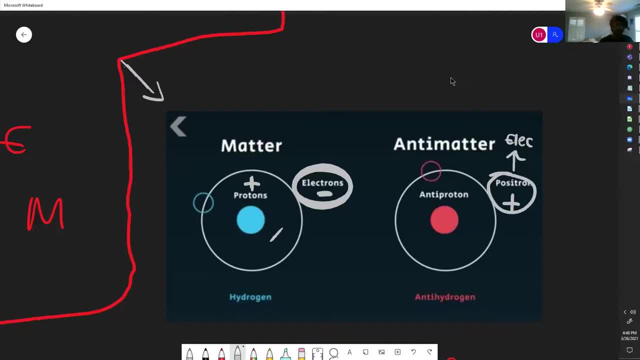 Positrons and electrons are the opposite in charge, But they share the same properties as they are not part of the nucleus And they are also have masses that are very similar. They have the exact same mass. Antiproton will be a negative. 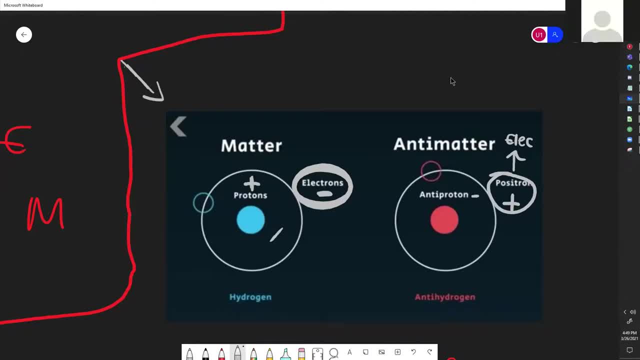 Yep, Good job, And that's kind of. that's kind of, yeah, So antiproton would be negative? Yep, Wait, what about neutrons? Neutron, the antiparticle of a neutron, it doesn't have a charge, right. 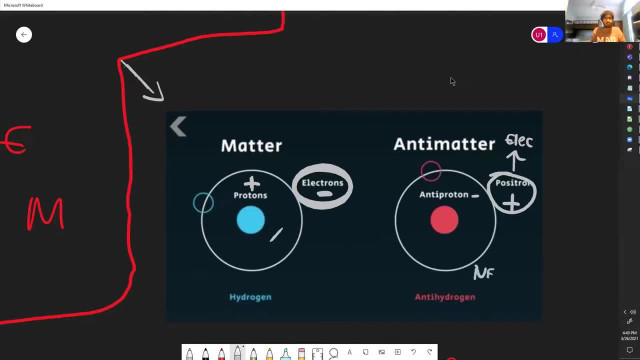 Because there's no opposite for neutral right. So the antiparticle for a neutron has the same mass and everything. It just has the kind of opposite properties And no charge. because there's no opposite for no charge. Yeah, So positron electron. 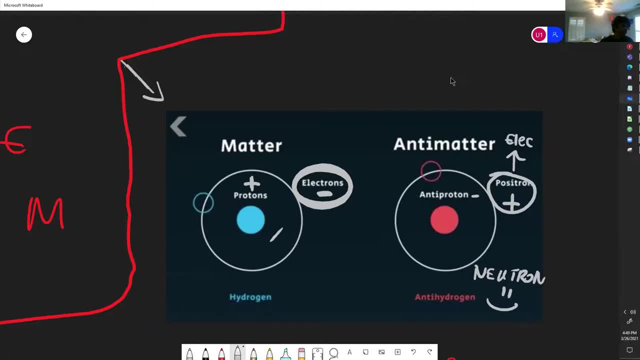 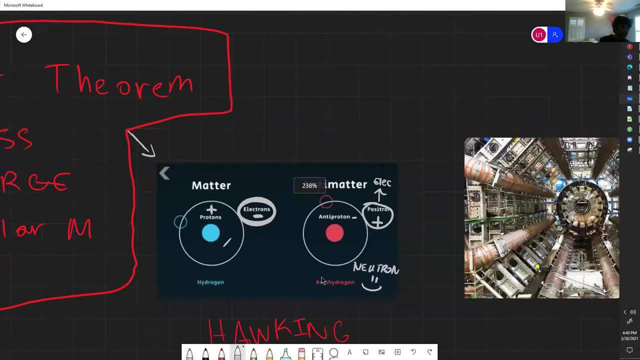 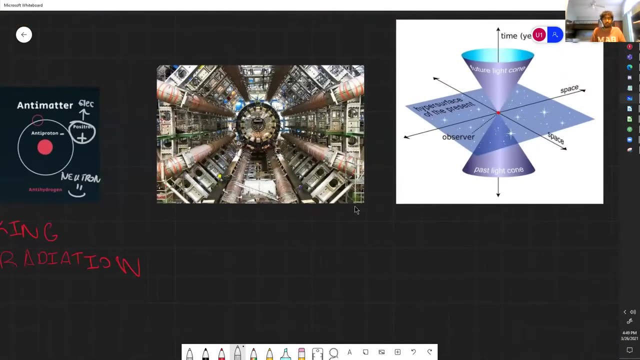 Antiproton proton Charges are opposite, But an antiproton is like a proton and a positron is like an electron. Bingo, Okay, Want to get into it. So antimatter can. actually, we have produced antimatter before, if you believe it or not, right? 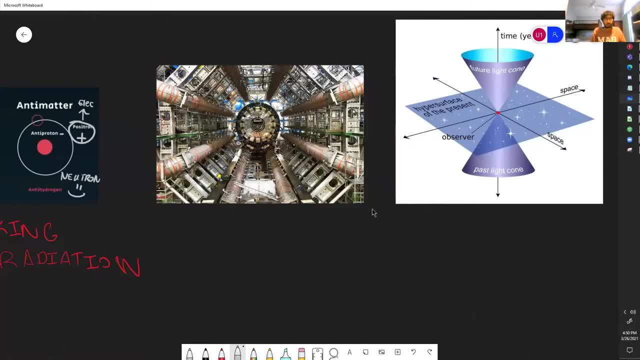 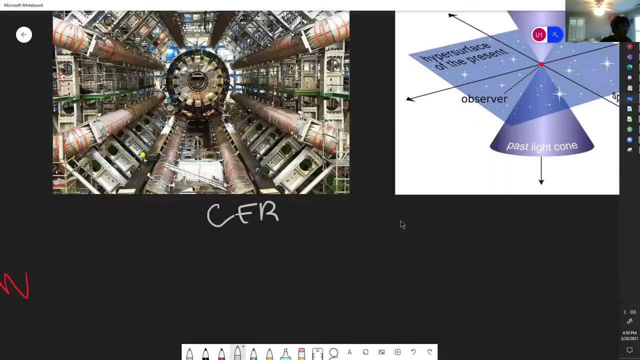 So has anyone heard of CERN? Well, to put it in, oh yeah, let's, let's run through this a little quicker. But CERN is. Yes, the CERN is the Center for European Research on Nuclear something, Nuclear physics or nuclear something. 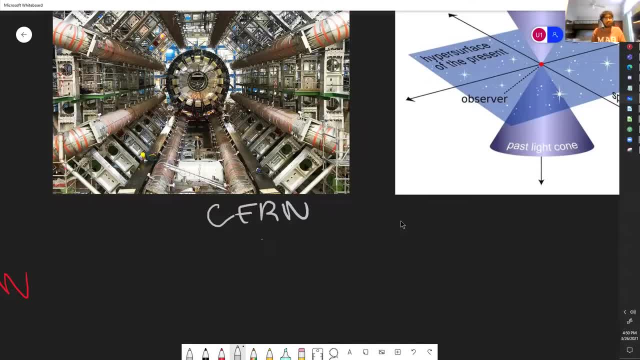 I don't remember the exact name, But CERN is like this. it's like a giant particle accelerator. What they do there is it's based in Switzerland, in Geneva, And they smash particles together and they discover all these kinds of new particles. 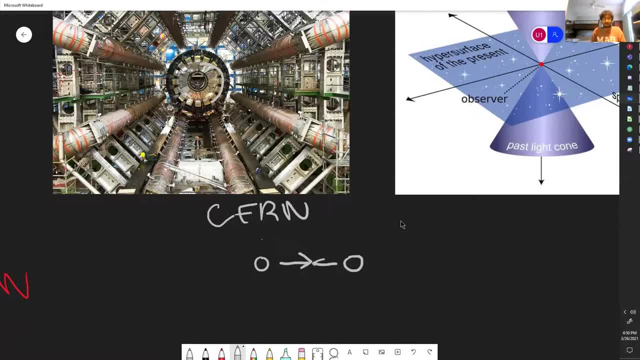 And they actually have a building called the Antimatter Factory where they have made antimatter before. I'm not sure how, but all I know is that they do. Now here's a. here's a small tidbit Might help you on the quiz. 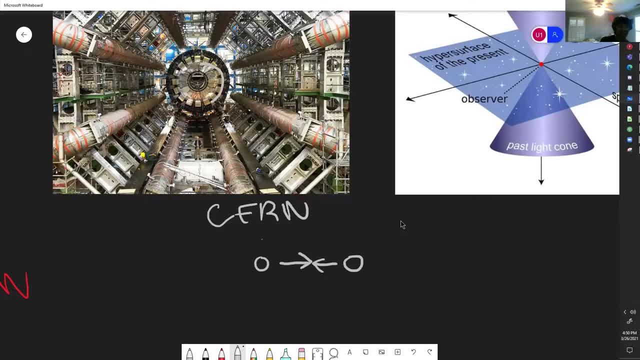 So with antimatter it's very. what do you think is going to happen if you go at and go to CERN and show up with a couple, a couple trillion dollars And it's like give me one particle of antimatter? 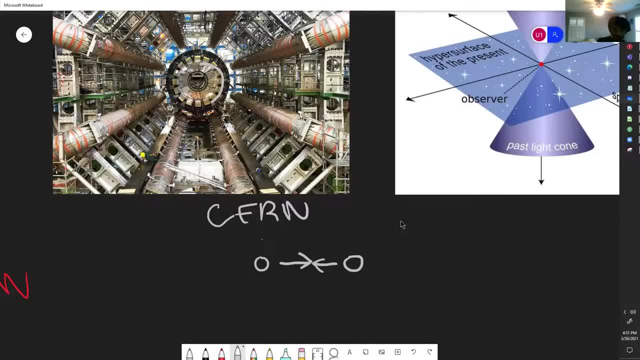 What do you think they're going to? what do you think is going to happen if they give you that one particle of antimatter? It's going to immediately annihilate itself. Yeah, So that one particle as soon as it meets with matter. 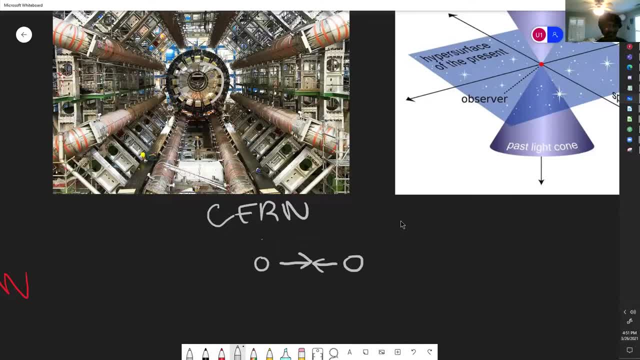 it is going to go kaboom. It goes kaboom, Like not even kidding. If you, if you put one particle of antimatter on matter, it is going to go kaboom And very bad. fun fact: Yep, The price of one gram of antimatter is $76 trillion. 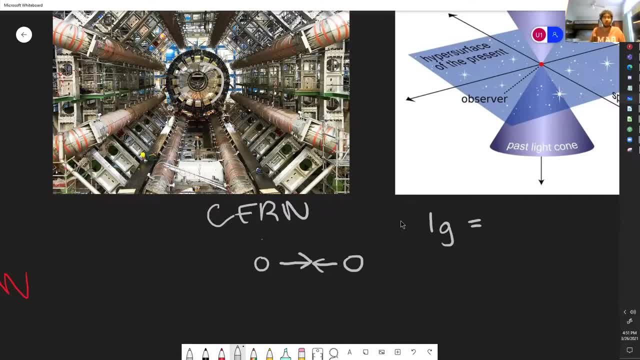 It's because it's extremely expensive to even create one particle Right And, in comparison, the entire world economy in one year. it's only about 20, I think 22 or $23 trillion. Yeah, Your question, Sanjeev. 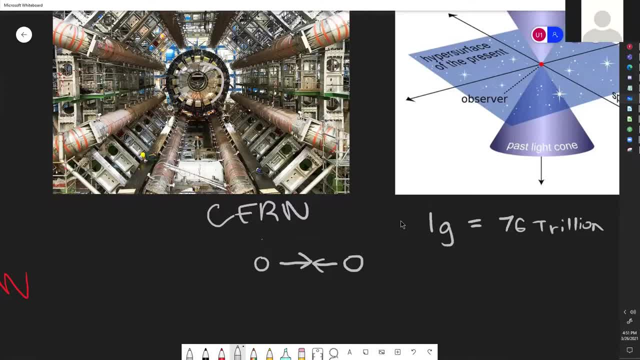 How do they store the antimatter if it just like goes kaboom when it touches matter? We don't know, We don't know, I don't know how they, I don't think they even tried to store it. I think it was just created and then it immediately annihilated. 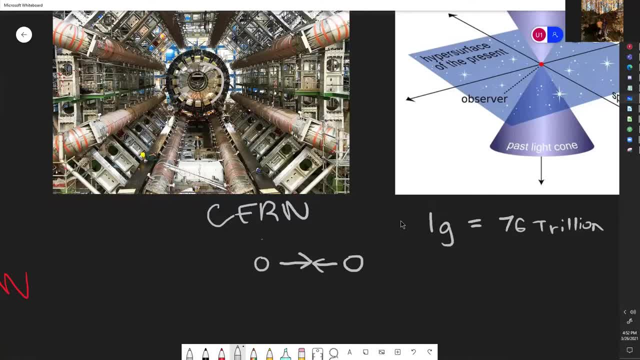 Do they contain it in vacuum? See, the problem with the vacuum is that you're going to have this, you're going to have walls to that container, the vacuum- But that antimatter meets the wall, it goes kaboom. If it touches the edge of the vacuum, the vacuum is kaboom. 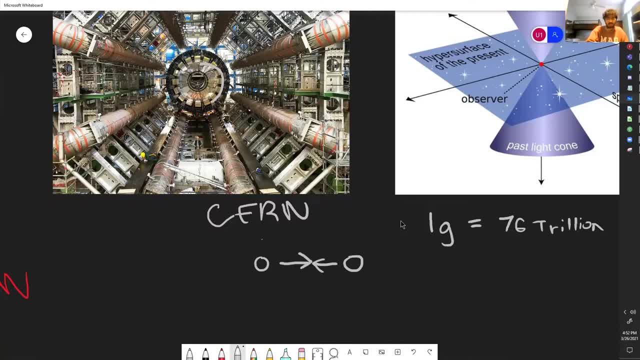 Exactly. Yeah. Well, what they could do is they could make the entire wall of the vacuum. They could make the antimatter with no position on and make the entire wall of the vacuum negative. I mean positive, no negative charge. 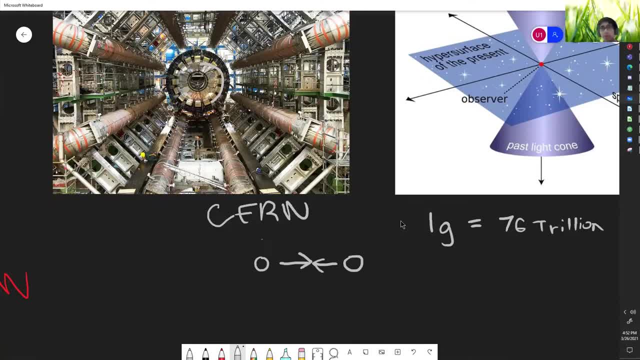 And then the antimatter is negative charge, So it won't touch the walls of the vacuum. That's really smart. Why don't you go work at Zoom? That's a really smart idea, Arv. Yeah, that's a really good idea.